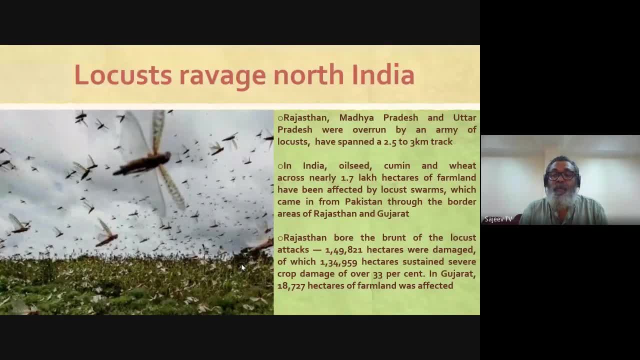 Many of the crops were affected. The Rajasthan had the most severe impact, with nearly 1,49,000 hectares of crop damage in Rajasthan And severe crop damages occurred in neighboring states, also with Gujarat. Nearly 18,000 hectares were damaged by the locust swamps. 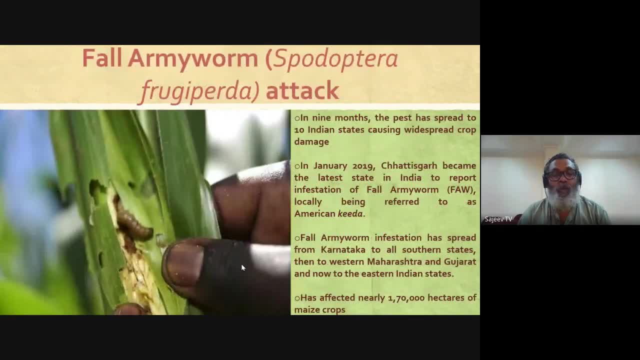 The following ones: the product of the frugipede attack which has happened in the past nine months. it has spread to nearly 10 Indian states- And such is good, which had the infestation in January 2019.. It has got a new report of this particular pest. 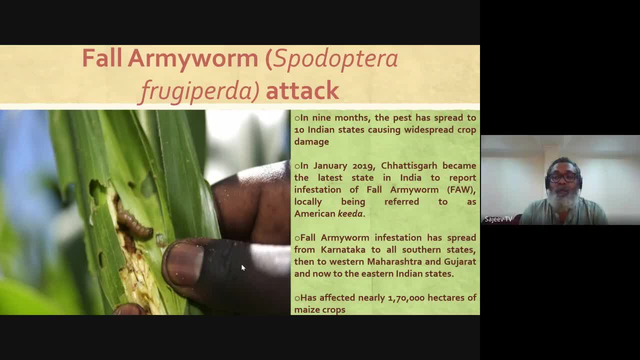 From the southern states, also from Karnataka. in Karnataka we had the very first outbreaks, which has spread to other states like Maharashtra and Gujarat, And now it is moving over to the eastern Indian states. Up to now it has affected nearly 1,70,000 hectares of maize crops. 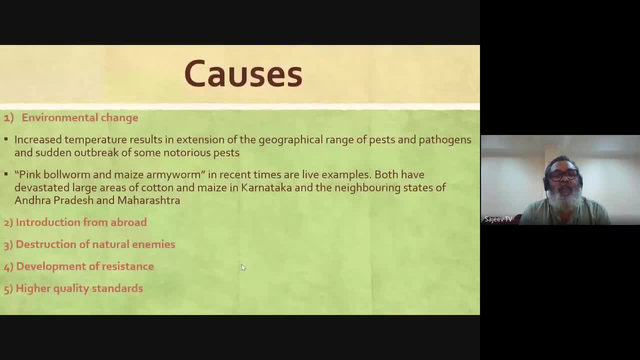 What are the causes of these big swamps of insects which come and damage our crops? Agriculture? There are several environmental causes which have been assigned: environmental change by way of increased temperature, resulting in an extinction of the geographical range of pests and pathogens. 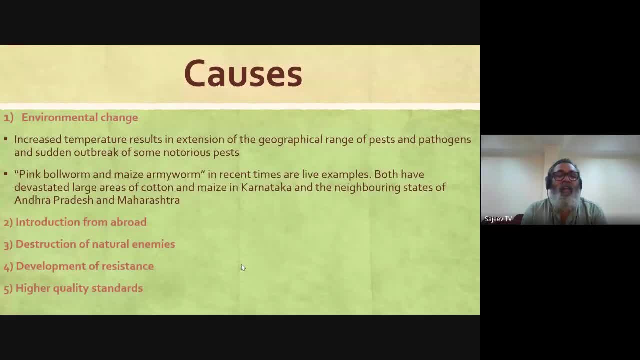 Basically, the lifespan of an insect is very solidly controlled by temperature. When the temperature increases, the lifespan reduces. So when the temperature is on the up there could be much more generations than in a normal year. One of the insects which I have seen 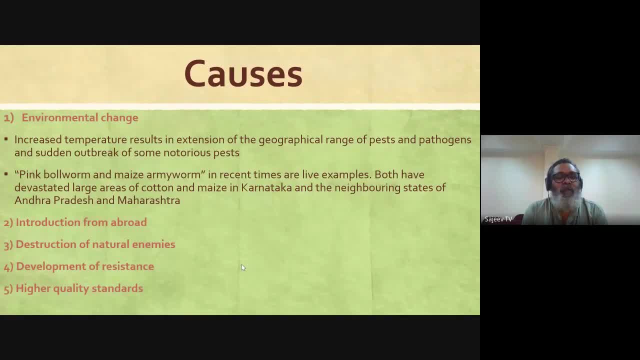 which I have studied, it normally goes to 13 and a half generations per year, But at an increased temperature it can go to 14 or even 15 generations per year. So when the number of generations increases, there is every chance that some of the generations 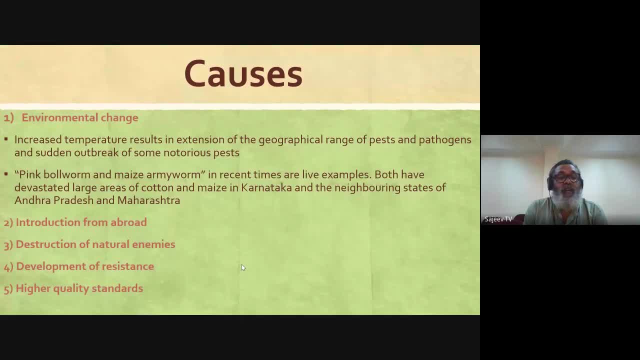 which have got good access to food can really cause an outbreak in the field. And another cause is the introduction of a new pest from outside. When that happens, there will be no local pathogens or natural pests. There will be no natural enemies of that particular insect right here. 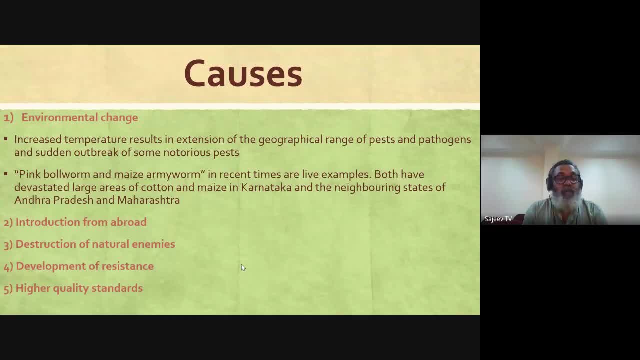 So there will be nothing to hold onto or control the population size and they become pests. And the third is that when you use chemical pesticides it kills the natural enemies also And the pest resurgence can happen. And the fourth is that many of the chemical pesticides 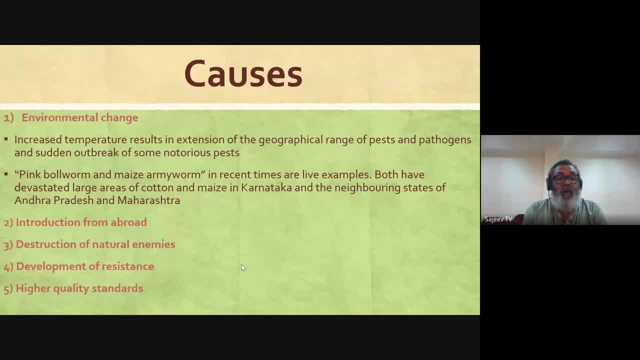 which you have been using can cause resistance for for the pest. And finally, we have higher quality standards which we have set up for many of the crops, especially the crops which we are exporting, which prevents us from using chemical pesticides. So it is difficult to manage. 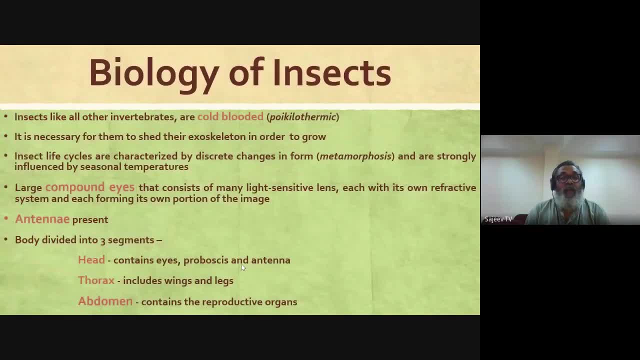 the size of the pests in the field itself And if you look at the biology, insects are basically called blooded, which is technically called organic organisms. They have to shed their exoskeleton in order to grow, a process which we call malting. 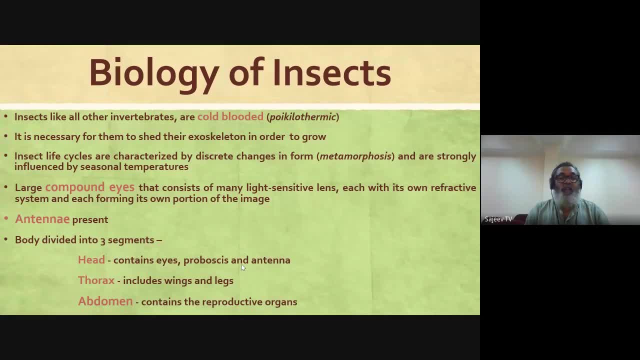 And you might be knowing about the metamorphosis which happens. And they have large compound eyes, which helps them to detect movement much faster- Agony, for instance, which helps them to detect chemical signals. And the general body is divided into the head, thorax and abdomen. 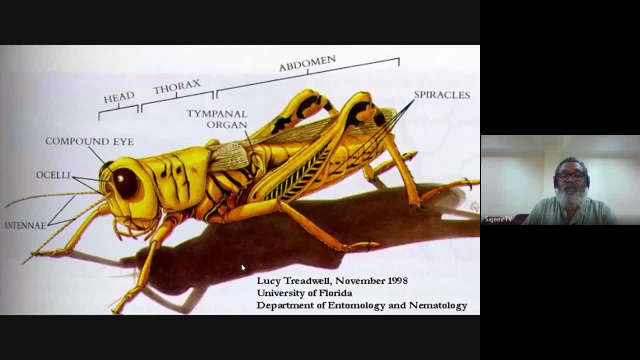 This is the structure of a typical insect. Here on the screen is a model insect from the group Orthoptera And basically this structure has been tested time and again and found that it is very adaptive to very different conditions. So I will not be going. 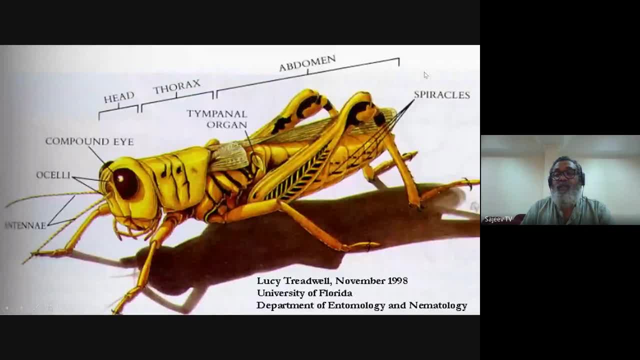 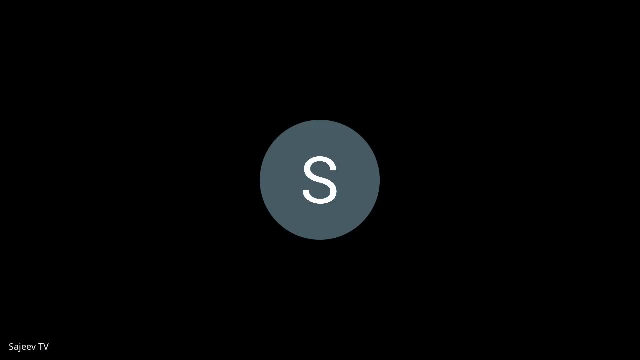 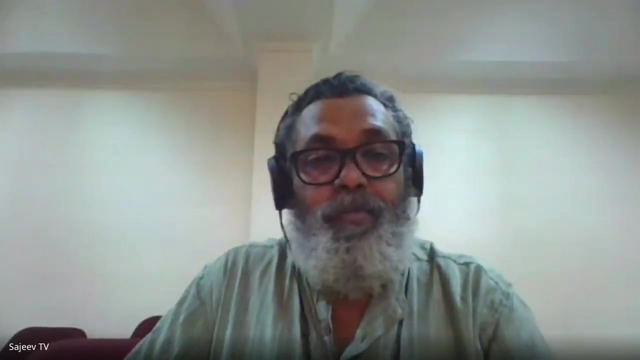 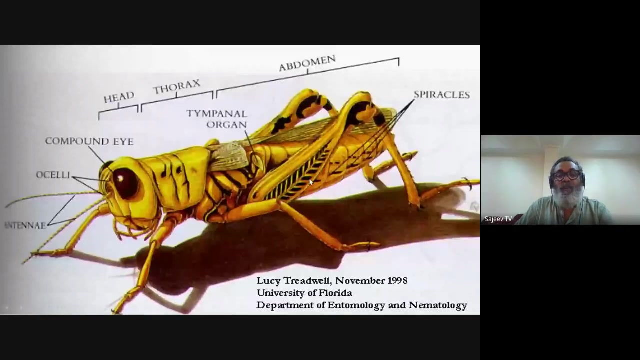 into the morphology of insects in a big way, But one thing which you need to look at is a thing called spiracles. The spiracles are small openings and they make the body bigger, And so that increases the efficiency- efficiency of it as an organism, So it can outperform many things than human beings. 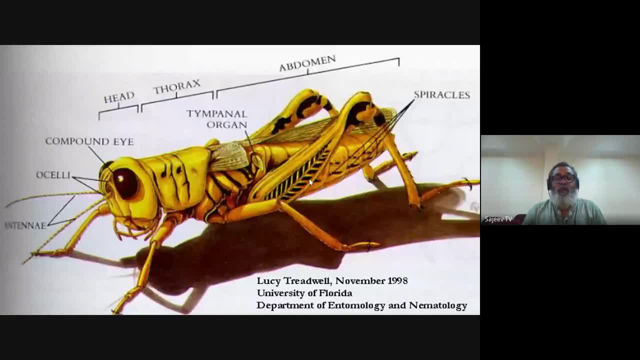 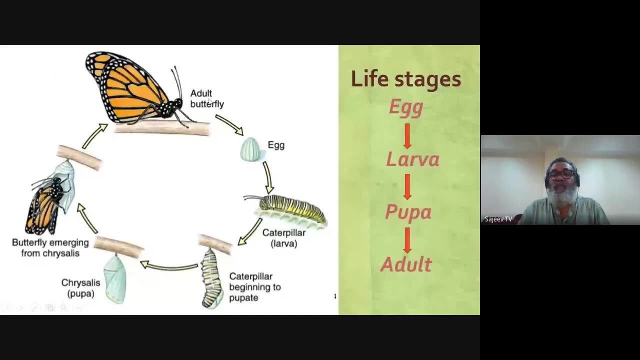 They can jump much longer distances than its body size. It can fly long hours. So all these capabilities are basically because of the intricate body design And the life stages where it's a complete metamorphosis happens. it goes from egg, larva, pupa and adult. 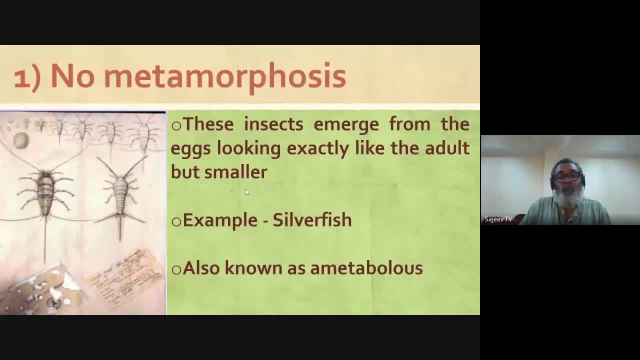 And there are other insects which doesn't have a metamorphosis also, For example, the silverfish which you find in your library, inside your books. they are also called as ametabolous. They don't go for a metamorphosis process. 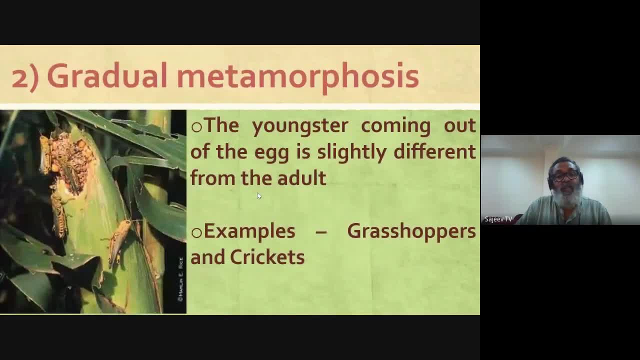 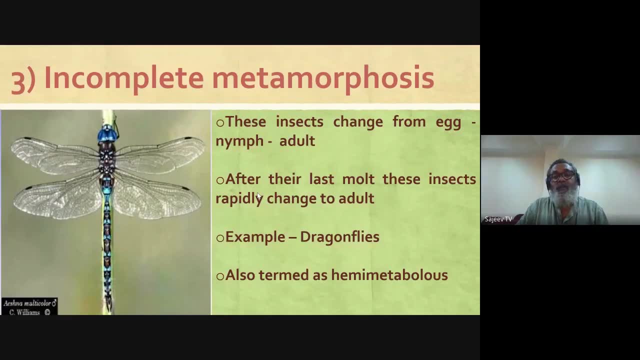 And there's other insects which go for a gradual metamorphosis, like the grasshoppers and crickets, And there are other cases with which there's an incomplete metamorphosis. There'll be only just three stages: the egg, the nymph and the adult. The pupae stage will be totally absent. 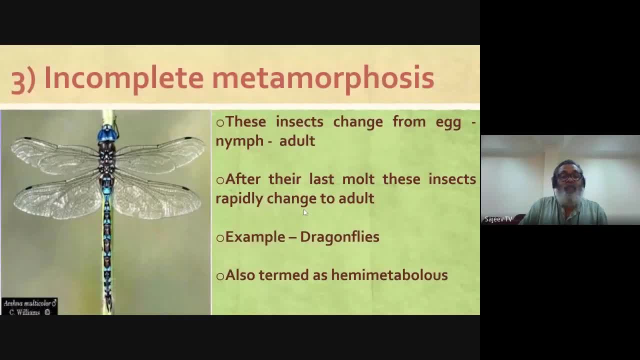 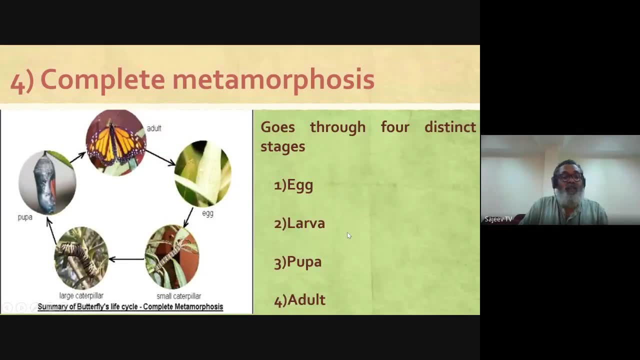 The examples are dragonflies, which are also called as hemimetabolous, And this is a complete metamorphosis which has got the four stages: egg, larva, pupae and adult. normally seen in most of the insects, including the butterflies, moths. 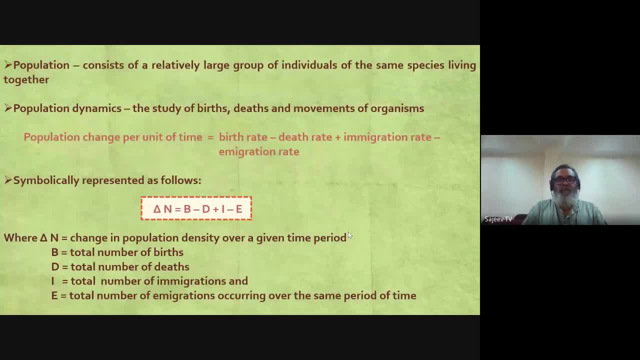 And the population is basically defined as a large group of individuals of the same species which lives together, And the population dynamics basically looks like the fluctuations of the size of the population, which is quantified in this particular equation. So population change per unit of time is equal to: 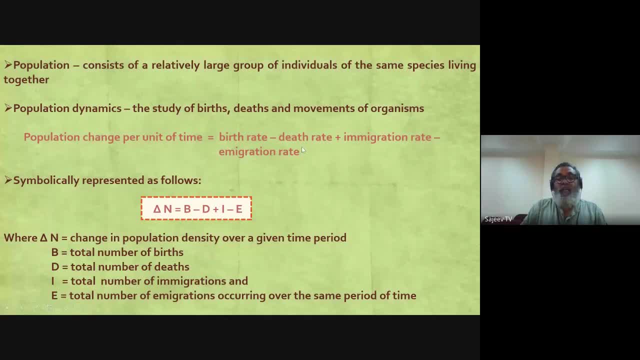 the birth rate, the addition of insects minus the death rate, the loss of insects plus the immigration rate, the number of insects which comes to a particular location minus the immigration rate, the number of instances which are left in the particular space, And it is as well as delta. n is equal to b minus d plus i minus e. basically, 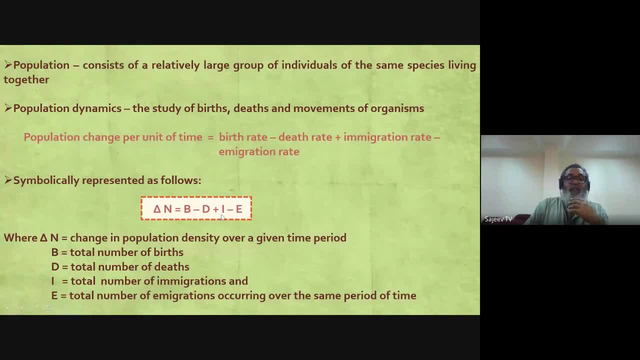 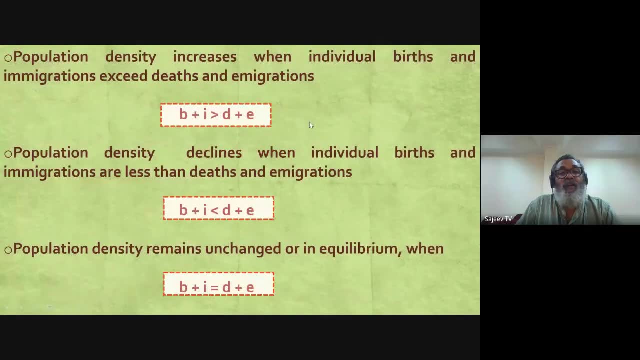 birth rate minus death rate plus immigration rate minus immigration rate. So what essentially this equation means is that the population density increases when individual births and immigration exceed the set of migration. So we can call this: from when b plus i is greater than d plus e, the population increases. So when b plus i is greater than d plus e, the population 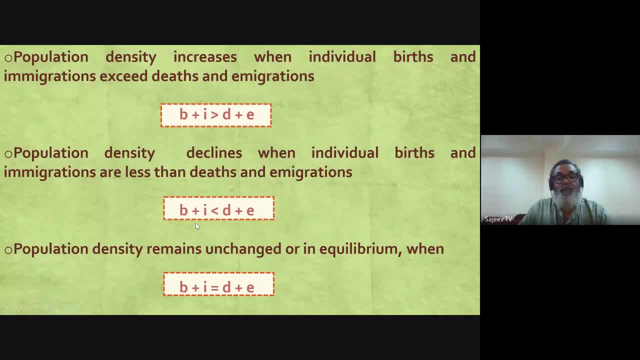 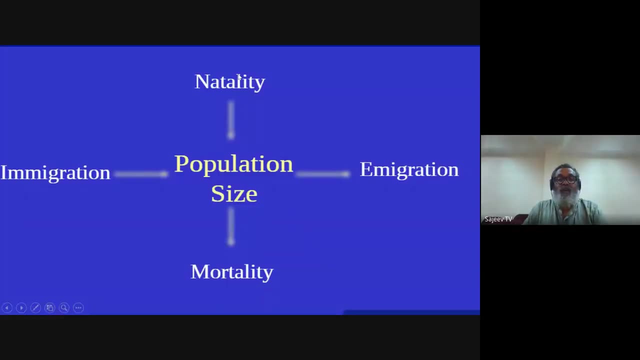 increases And it declines. when it is less from the birth rate and the immigration is less than the death rate and immigration, the population decreases And if both are the same, the population remains in an equilibrium. So this is a relationship. It's a natality- mortality. 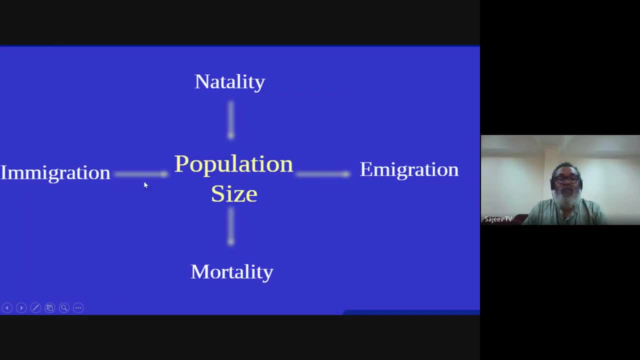 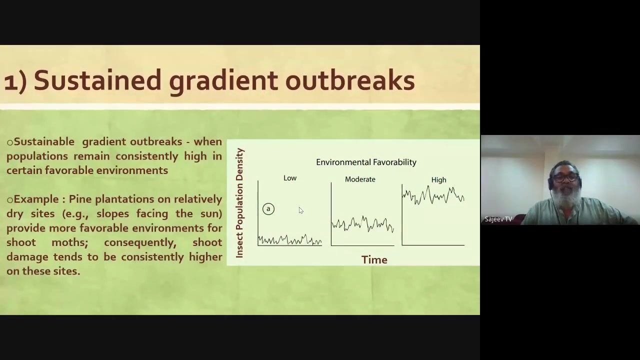 immigration, immigration. So natality adds to the population size, immigration adds to the population size, mortality reduces the population size and immigration also reduces the population And we have the theoretical concept of population. dynamics have classified insect outbreaks into many different categories, And this is the first one, the sustained gradient. 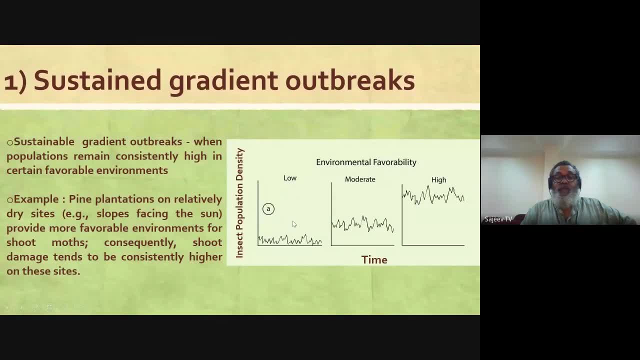 outbreaks when populations remain consistently high in certain favorable environments. So this is a low level, where an insect population density is plotted against time, And this is a moderate one. and this is a high level. The population remains at a particular level continuously for a 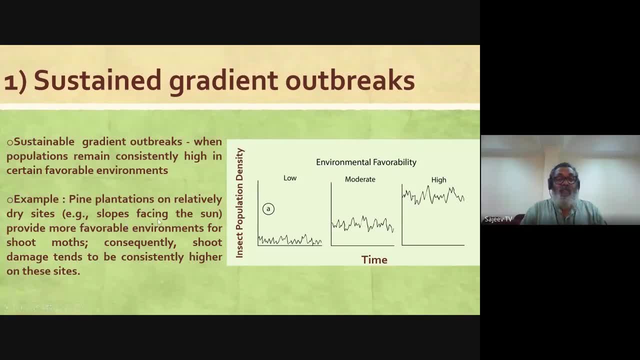 period of time. Example is the pine plantations on relatively dry sites. They have a favorable in long for short mass. Consequently, shoot damage has to consistently higher on these sites. So when that happens, the impact will be consistent and remain for a long period of time. 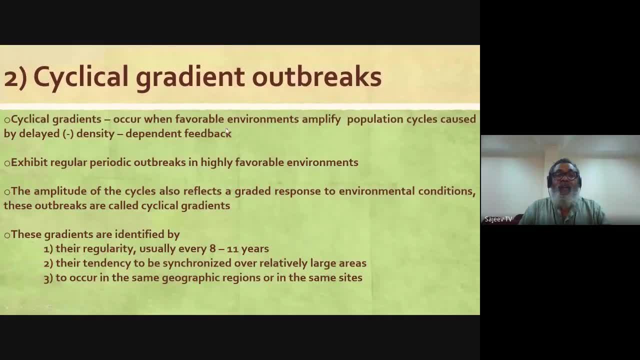 The second is a cyclical. graded outbreaks Occur when favorable environments amplify the population cycles caused by delayed, density-dependent feedbacks, And they exhibit regular, periodic outbreaks in uh environments. uh the uh. they are basically cyclical. they reappear at a particular period of time. for example, there are. there's a regularity usually. every eight to eleven years you get a big buildup of the population and uh their tendency to be synchronized over relatively large areas. they get synchronized, uh they. normally this cycle happens in the same location at uh regular uh intervals. they do not spread far from the points of origin usually associated with the defoliating, insisted lip. 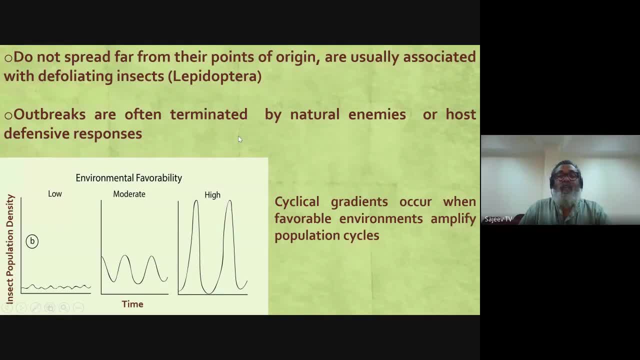 adapter. uh, these outbreaks are normally terminated by natural illness or horse defensive responses. and this is a way it happens: uh, environmental favorability uh, when it increases, uh, the insect population uh moves to a particular cyclical pattern. so you have a big outbreak over here, it collapses and then it again happens, and 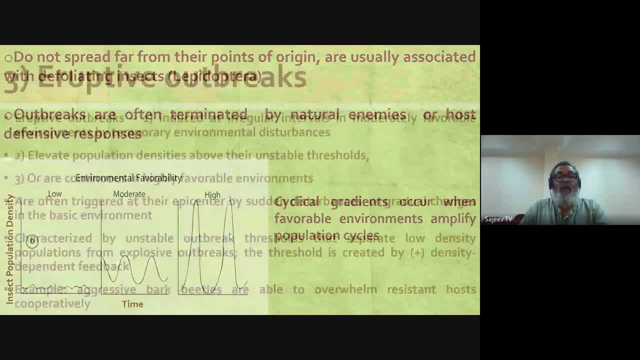 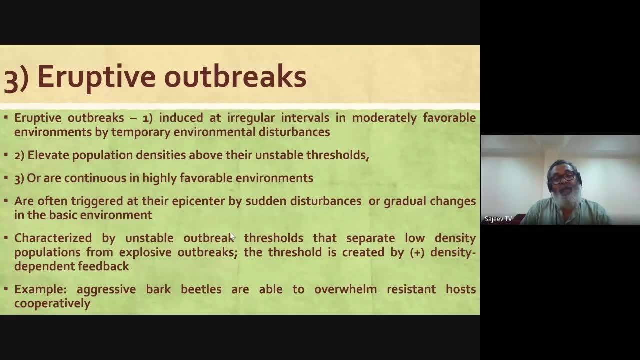 this becomes a cyclical phenomenon and then we have the eruptive objects uh. they are induced irregular intervals by the cyclical outbreaks where the uh regular uh in frequency. these eruptive outbreaks are irregular and they are caused by temporary changes in uh environment and they uh. 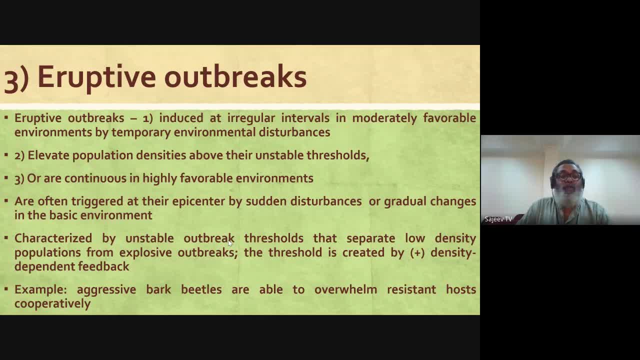 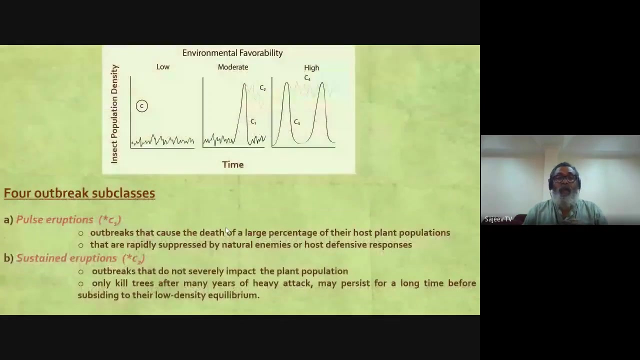 the population density is above the unstable thresholds or a continuous in high favorable environments, uh they. whenever there is an eruptive outbreak, we normally observe an epicenter, a small place where there's high intensity uh insects, uh density of insects, which uh erupt from there and spread to larger areas, causing outbreaks. and this is how it happens: there's a lower level and then 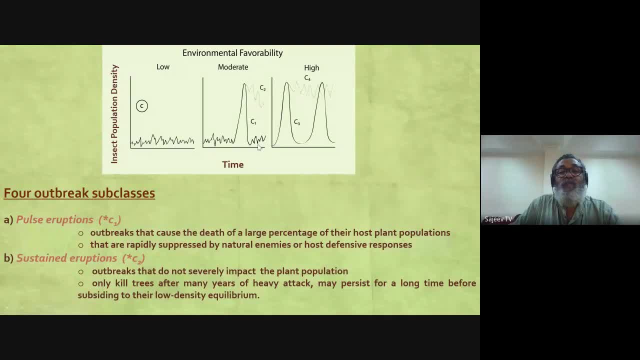 there's a moderate level at which you get a outbreak once in a while and then it sustains uh, but then, unlike uh, either you can go up and sustain at a high level or it crashes and then come up again. but this, uh, this is a quite a regular uh thing, uh, and when it happens, uh. 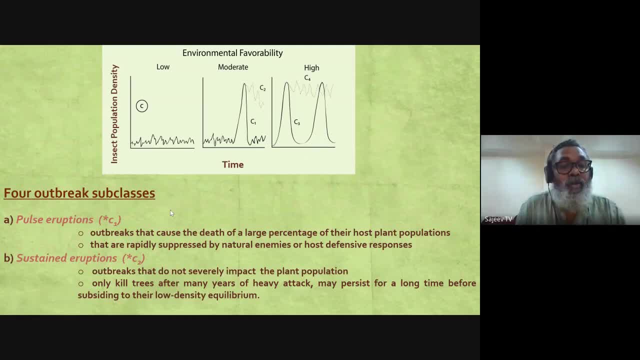 uh it it have. it is classified into two or uh, two types of which are outbreaks that cause death of a large percentage of their host, a plant population, and they are rapidly suppressed by natural enemies. this is. there's just one pulse uh which is happening. it should be completely uh uh. 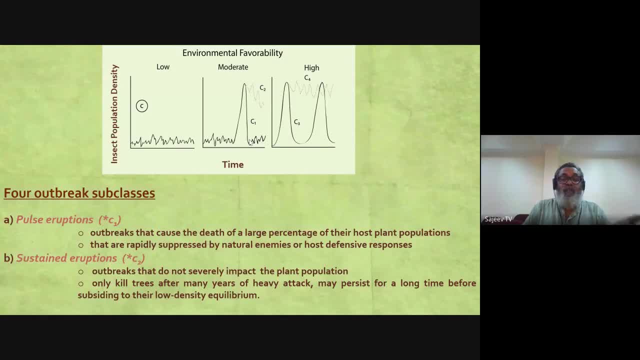 managed by the response of the host organism or by the increase in natural enemies. but then there could also be sustained eruptions. eruption happens, happens, and then it gets, uh, sustained for a long period of time. so this is going to be much more impactful on the host plant. 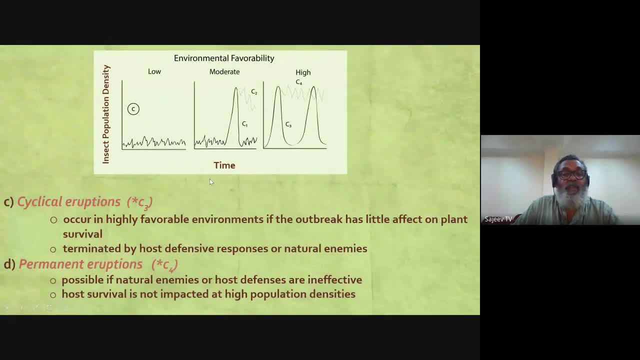 and uh. we have cyclical eruptions, uh, which i have told you earlier, and there are permanent directions. possibly, if natural enemies of holdings are completely ineffective, like, for example, for invasive insects- instances which has come to us and have created a problem- without the uh natural enemies over here, they can sustain the eruptions which has happened. and uh, you come to. 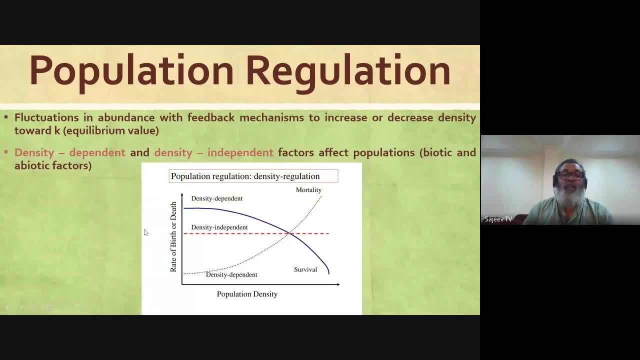 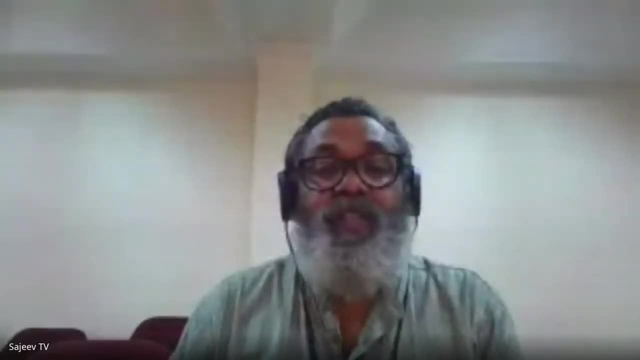 population regulation. how is the normal, normally the population regulated? uh, in the environment feedback mechanisms to increase or decrease density. to where the k? so basically, there are two different types of population regulation which happens. one is the density dependent regulation. so when the density is very high, uh, it is not sustainable it. 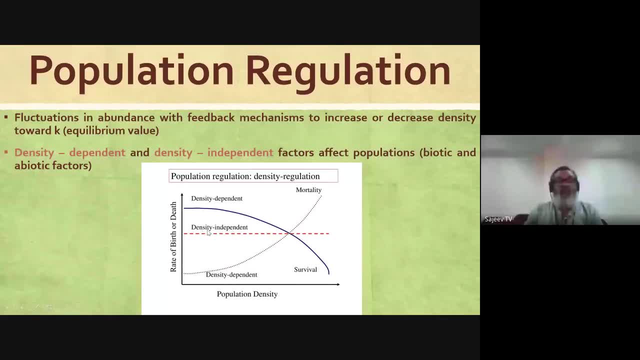 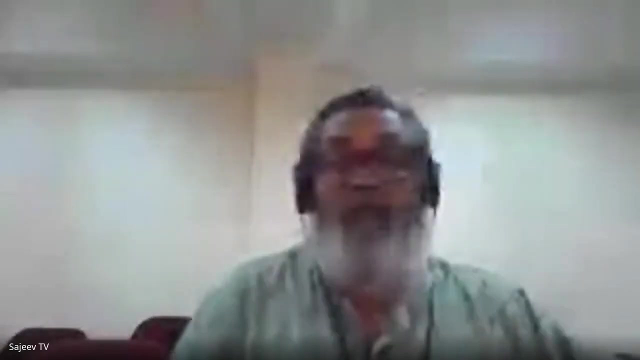 goes down. and then there is the density, independent of regulation, where the regulation, if it happens, is because of abiotic factors like temperature, humidity, rainfall etc. and it is not based on the density of the. it is not related to the density of the insect. so when the rate of birth or death increases, it causes a large level of impacts and 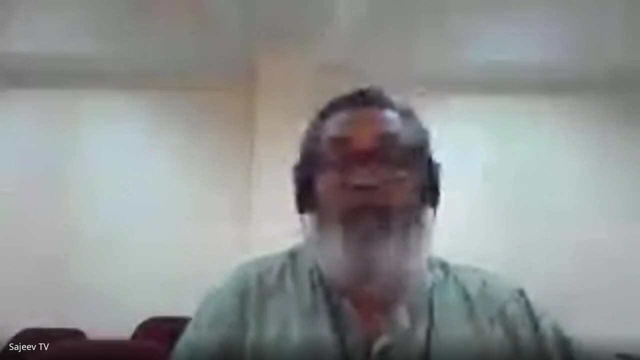 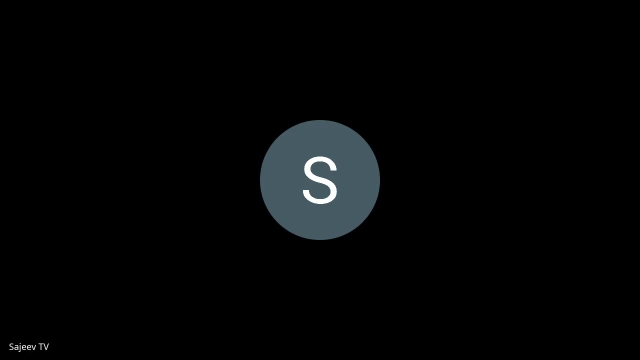 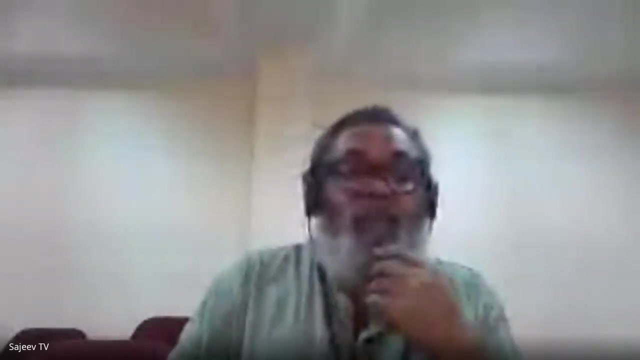 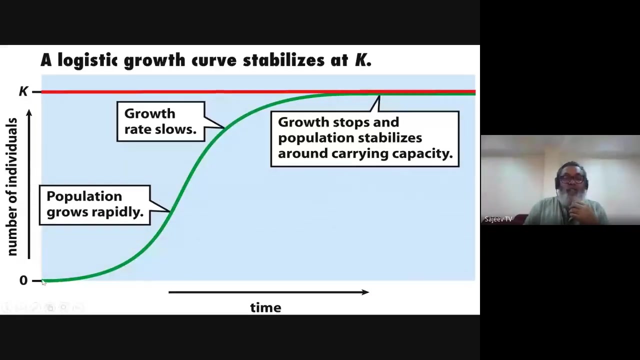 the crash can happen, but it can also increase when the density dependent factors, the factors which affect the population dynamics, are on the decline. normally this is what happens: the number of insects when it go towards the carrier capacity it reaches when the population increases from here, initially the population grows rapidly and then the growth rate slows down, it reaches a plateau. 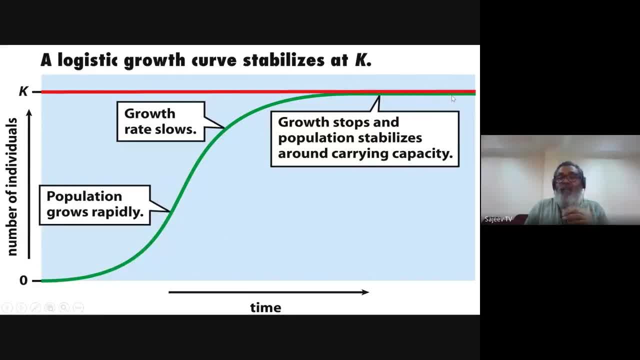 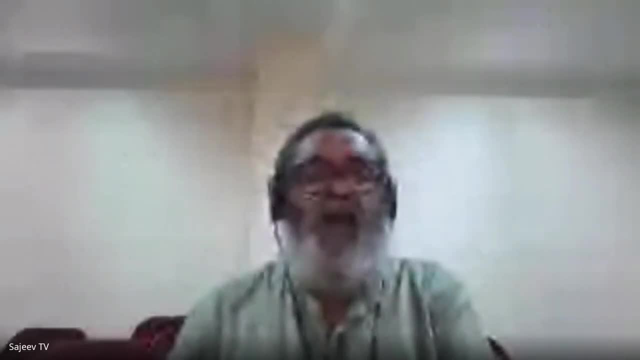 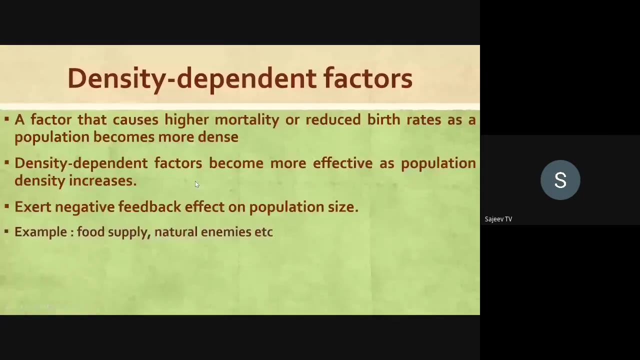 and the growth stabilizes around the carrying capacity of that particular population. now the next one is the density dependent factors, a factor that causes higher mortality or reduced birth rates as a population becomes more dense, and there could be two positive feedback loop. these are some examples of the density independent effects, like when the 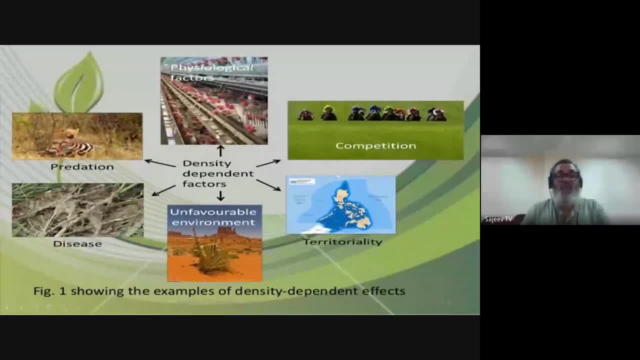 density increases, there could be physiological factors which work against it. there could be competition, which is happening, there could be a territoriality which, uh, which completely, uh, uh, rustic, the population and, uh, the environment becomes unfavorable and disease could happen when, when the density is very high and there's a you know, 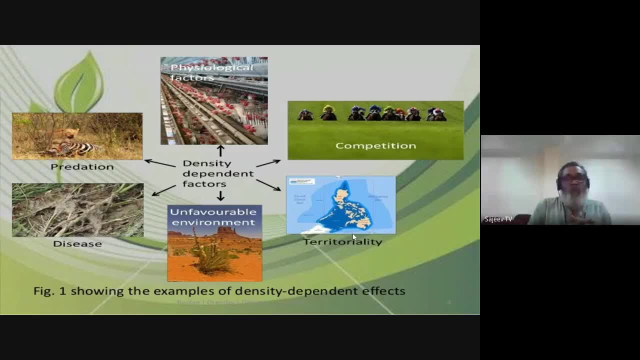 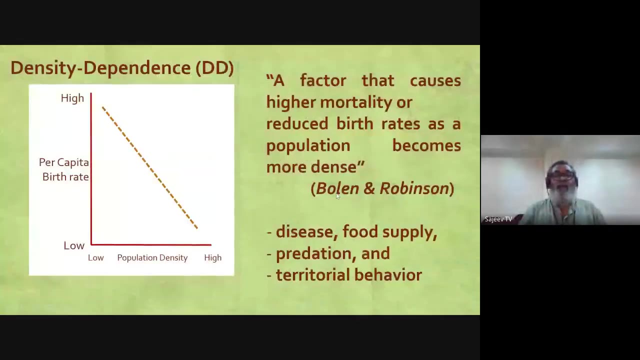 incidence of a disease. it spreads very fast and predation will also increase. because there is large amount of prey, it is easy for the predator to uh to access it. so these are the density dependent factors, which reduces the population size, and the density dependence factor that causes higher mortality or reduced birth rates as a population. 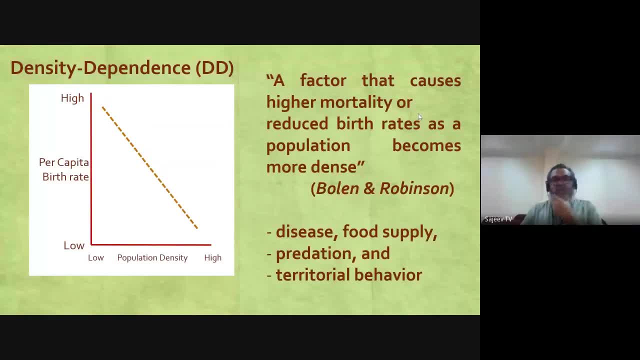 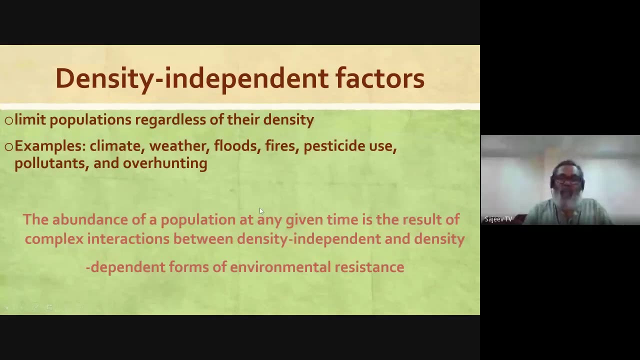 becomes more dense. that's what's called the density dependence. it could be uh disease. so, as i told you earlier, uh the supply of food, the predation and territorial uh behavior and we come to the density independent factors. they limit populations regardless of the density uh. the examples are climate weather, floods, fire, pesticide use, pollutants and overhandering. 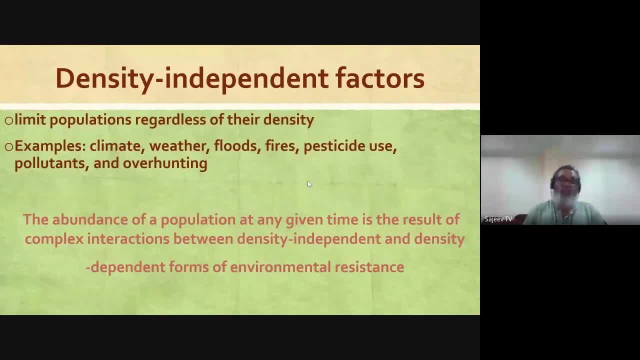 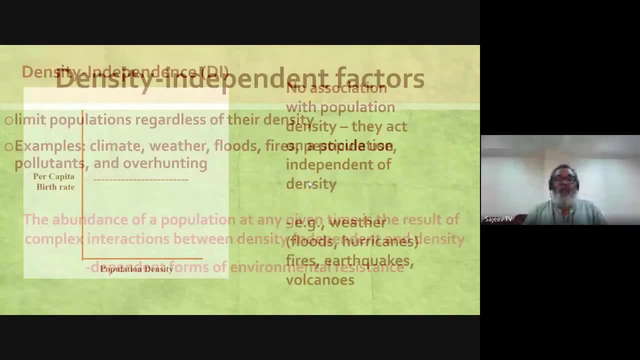 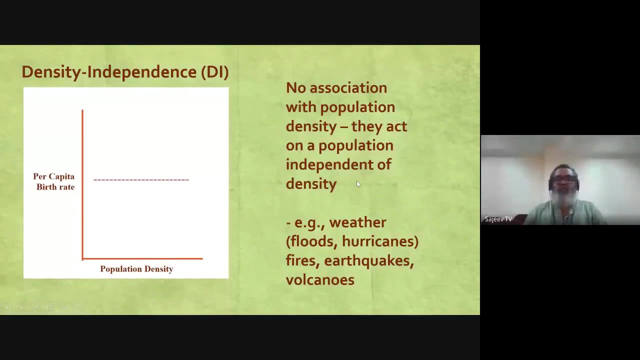 so basically, there are two different ways in which a population is regulated. one is the density dependent factors and the other is the density independent factors. there's no association with population density. they act on a population independent of the density. so this is basically the theoretical structure. i would like to also introduce this. 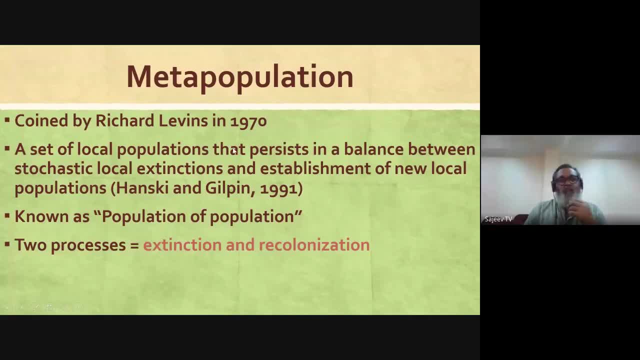 term called mature population. it was called by richard levins in 1970. it is defined as the set of local populations that persists in a balance between stochastic local institutions and establishment of new local populations. a meta population is a group of different populations between which there is movement of organisms happening. so what it essentially means that a 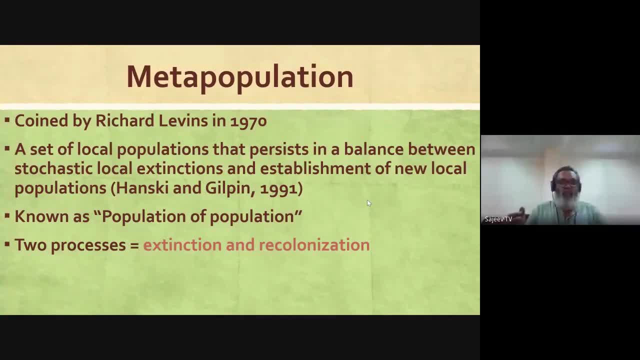 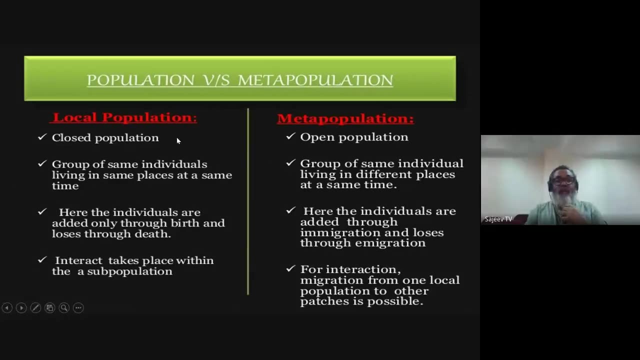 local population can either go extinct or a new place can be, uh, re-colonized, but the metal population remains almost stable, while the local populations are very erratic- we'll come to the practical implications of that later- and the local population is basically closed one, while the 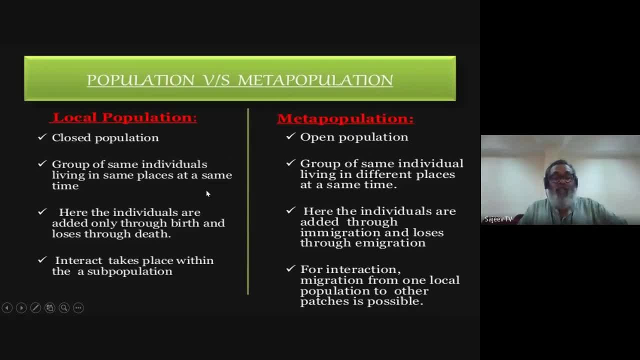 better population is open population, so group of same individuals living the same place at the same time is constitute the local population. while the group of same individual living in different places at the same time, those better populations have much more especially big uh space in which there are different populations uh living together. uh in the case of local populations uh the 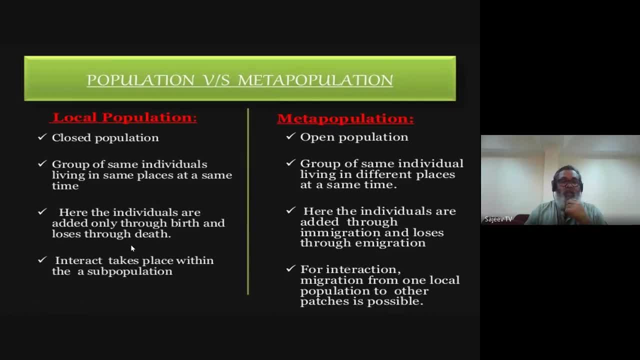 are added only by birth and lost because of death. In the case of metapopulation, the individuals are added through immigration and the loss is through immigration. So the interaction in the case of a local population happens within that particular population, But in the case of metapopulation, 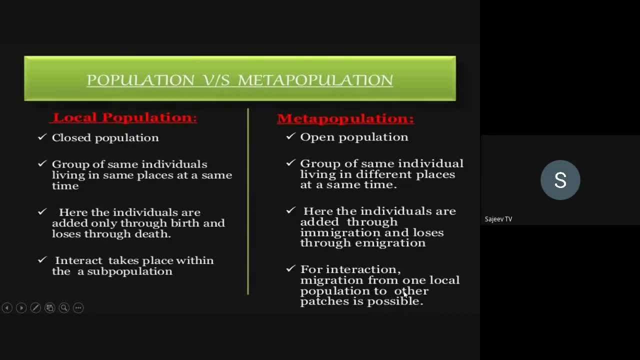 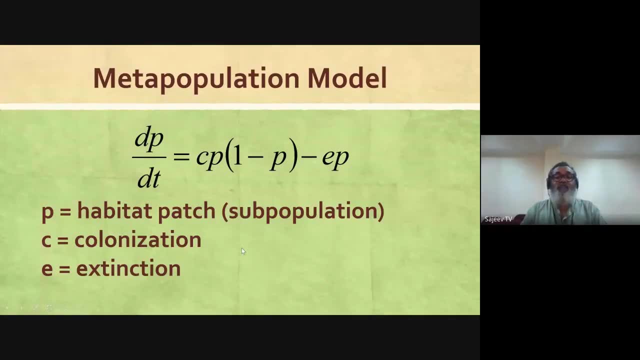 migration from one local population to other is possible, And this is basically the metapopulation model. I'll not be going to the details of that right now due to a paucity of time. So this is a basic structure of a metapopulation. 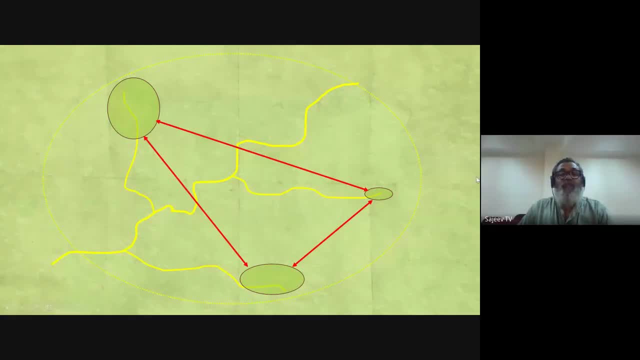 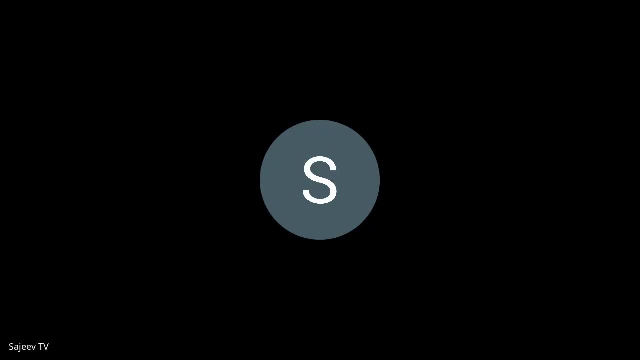 It's a local population. There are three local populations over here, but there is movement happening of individuals across the populations And we call the bigger structure as a metapopulation For the metapopulation. the first one is that the species has local breeding populations. 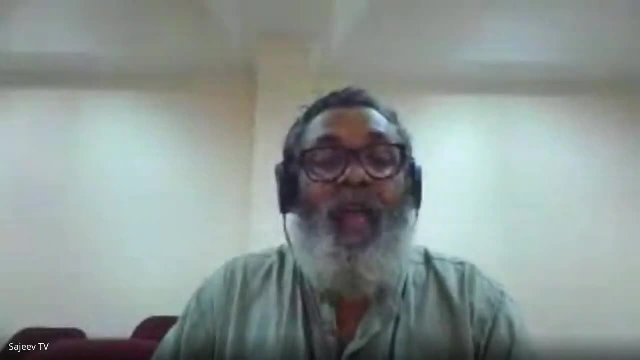 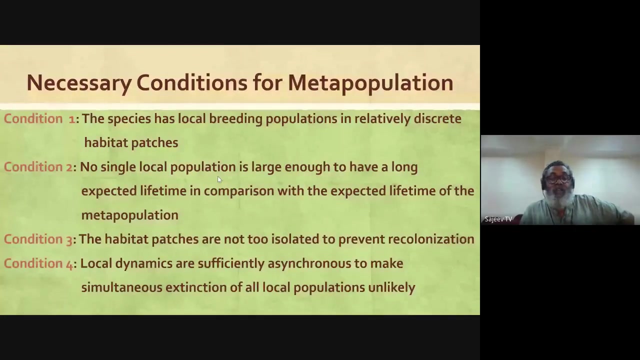 and largely district habitat patches. And the second is that no single local population is large enough to have a long expected lifetime in comparison with the other species. So this is a basic structure of a metapopulation. So this is a basic structure of a metapopulation. 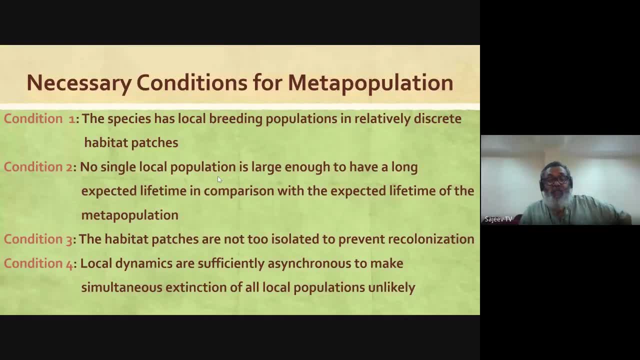 Thirdly, the habitat patches are not too isolated to prevent re-colonization, Which essentially means that there should be a possibility of movement between the local populations. And the last condition is that the local dynamics are sufficiently asynchronous to make simultaneous extinction of all local populations unlikely. 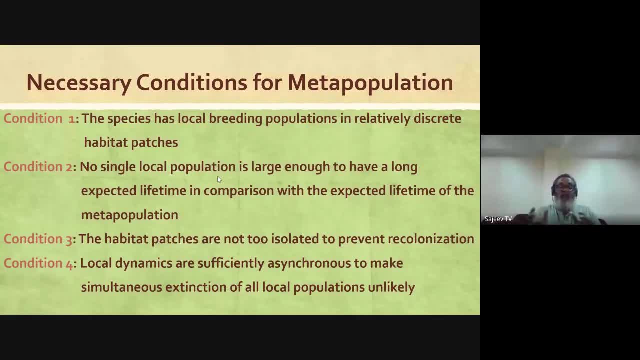 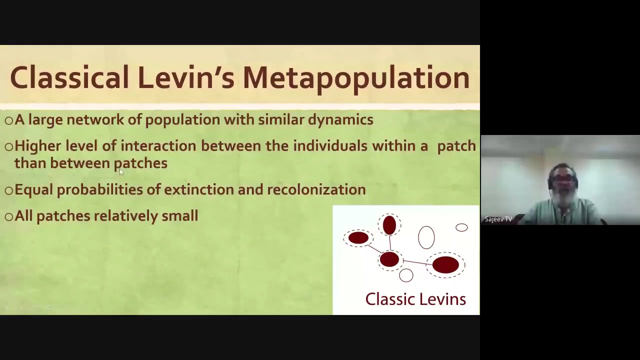 It essentially means that all the local populations should not be synchronous and should not go to the same place or go extinct all of a sudden together. There should be a sufficient asynchronous dynamics present so that, even if one local population is extinct, others survive, And these are some of the classic metapopulation models. 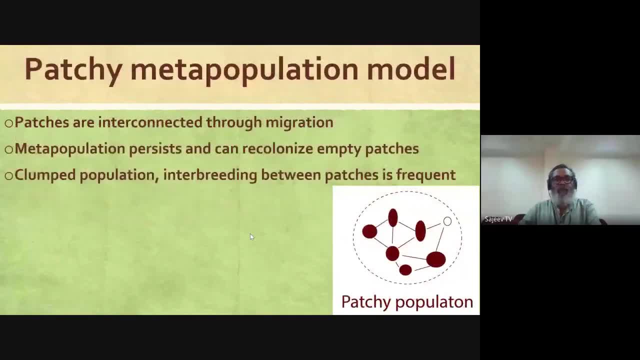 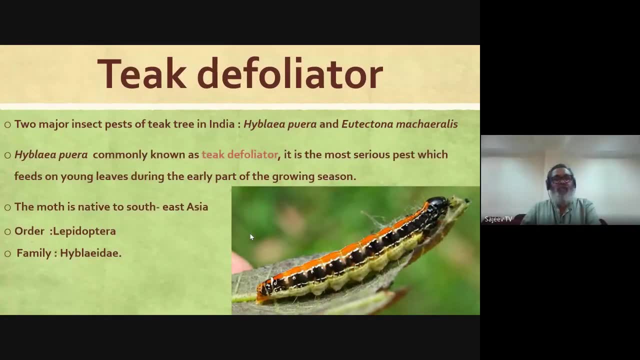 I'll not be going to the details of that right now. I'll come to one of the models which I had been working on, which is the T-defoliator. This is an insect called the Hiblia pura. It's a lipidopteran moth. 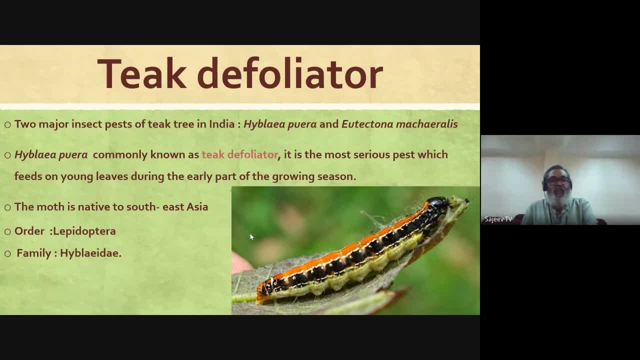 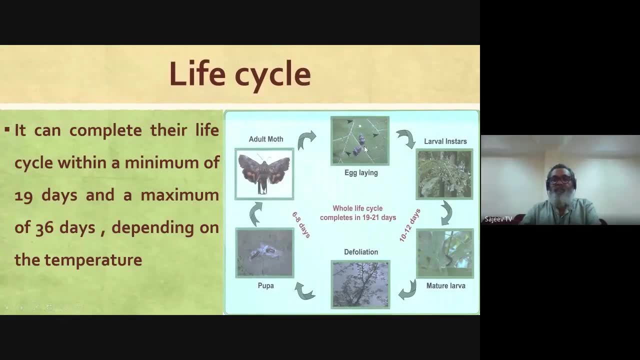 which is mostly seen in Southeast Asia. And this is the life cycle. It has got this egg-laying process which happens on the tented T-leaf foliage And it emerges into larval insters And it molds. there are five different larval insters. 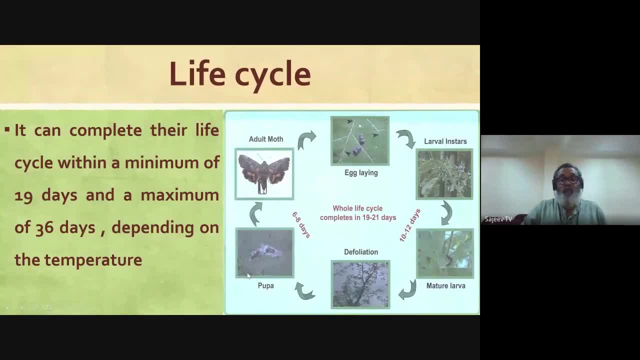 which causes the defoliation of the T-tree, And then it pupates on the ground. And if it's a remedy period, it pupates by folding the leaf of the plants which are living under canopy And then it emerges in a beak, it emerges to the moth. 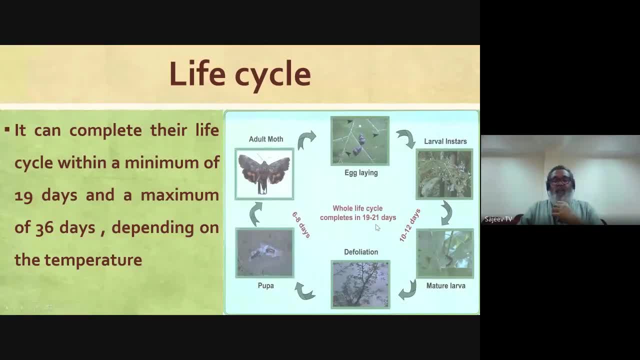 The whole life cycle completes in 19 to 21 days And small changes can happen based on the ambient temperature, And the minimum number of days is 19 and the maximum is 36.. We have compared the lifespan of insects in Nakedla. 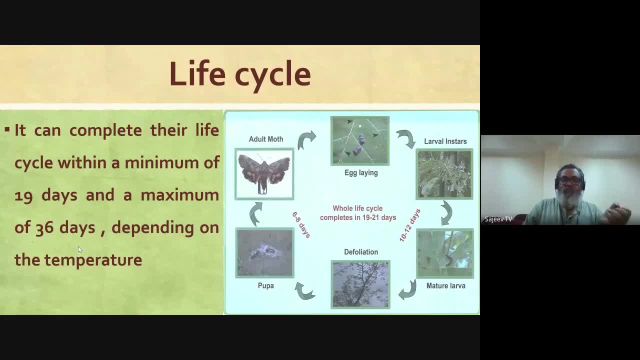 in Bangalore and in Dharadun, Three places with different temperature regimes, And we find that the Dharadun population took 36 days for completing one generation in 19 days And the ecological relationship set: this is Olicophagus it has got. 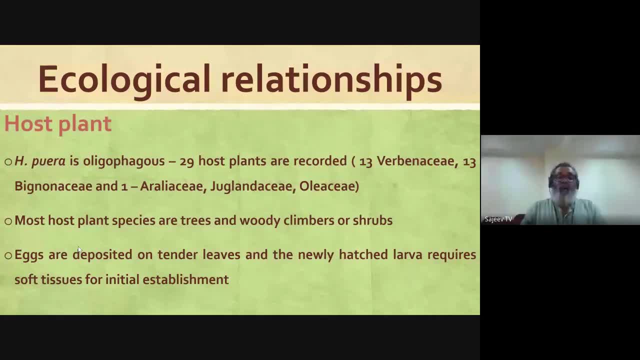 it feeds on nearly 29 host plants, And mostly they are trees, But a teak is a major host in the sense that teak plantations are extensive. In Kerala we have more than 75,000 hectares under teak, So there's enough food supply available for this particular. 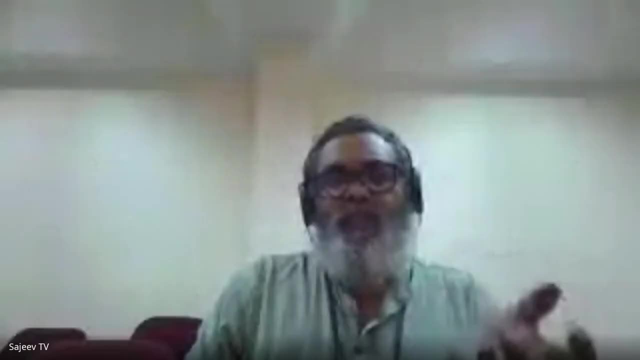 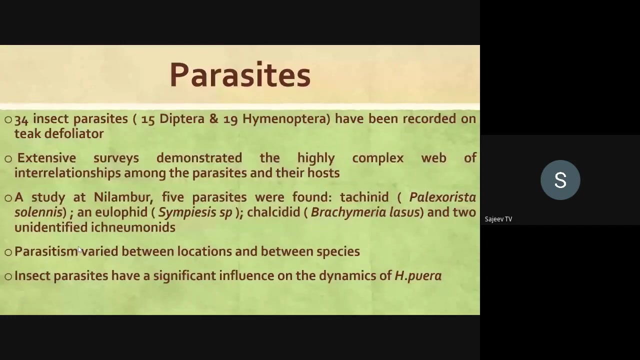 for this particular insect And looking at the natural, our predators, it has got 34 insect parasites, including 15 from the Dictoran group and 19 from Hymenopteran group. has been a partner for the teak defoliatum. 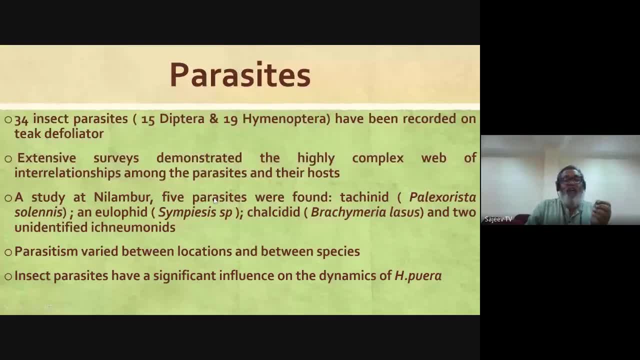 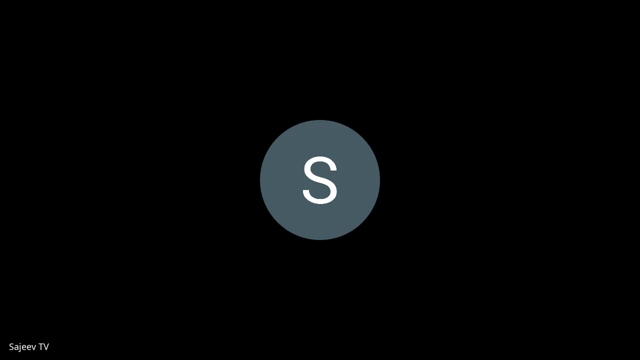 There's a highly complex web of interlation between the parasites and the host insect, And the insect parasites have a significant influence on the dynamics of Hibliopura during the non-hour period. The predators- in this particular it has a large case- the bats. 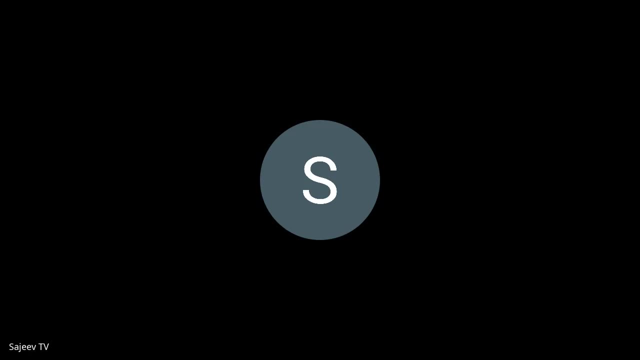 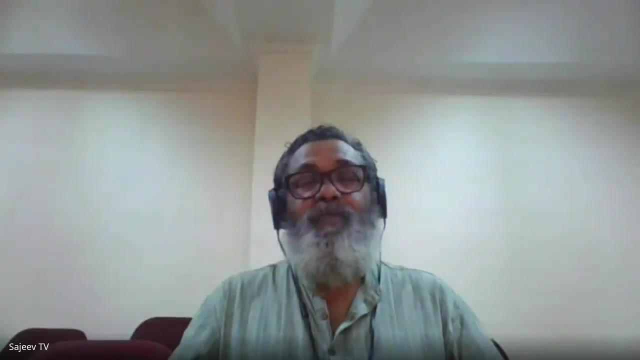 There are many predator species And there are pathogens also. There are two bacteria had been identified. One is, and the other one is the Enterobacter aerogen Aargh, and will be found on the top branches in an inverted V shape. 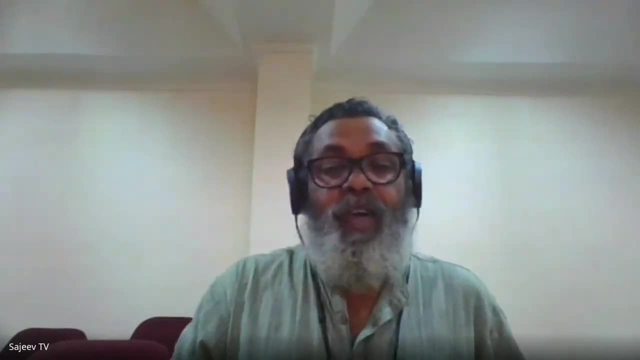 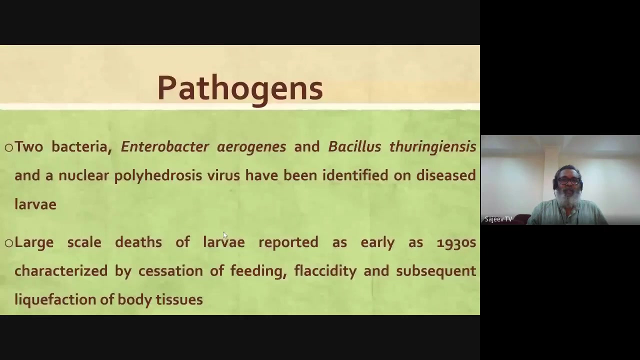 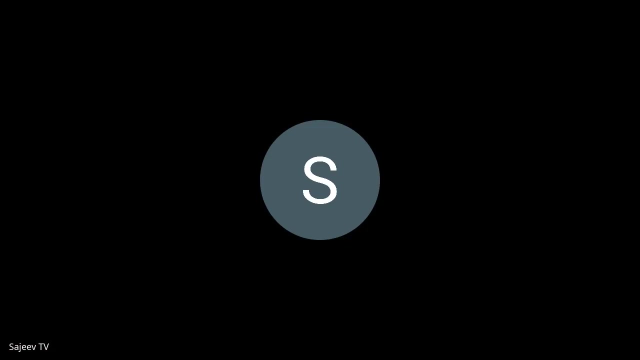 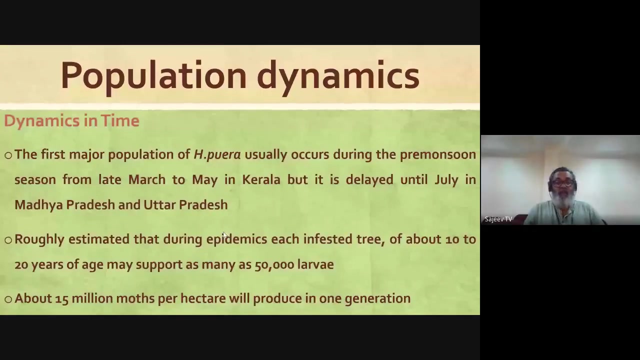 So that's a classical symptom of a virus induced death in a moth And when you come to a couple of the population in Kerala. But it's delayed until July in the center part of Kerala and the northern parts of India And we have a very small episode list to start with which expands to bigger areas in every. 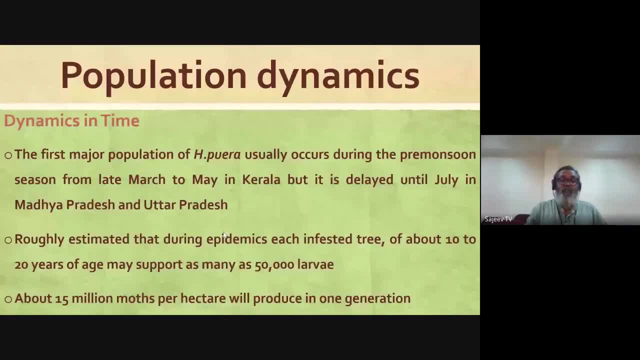 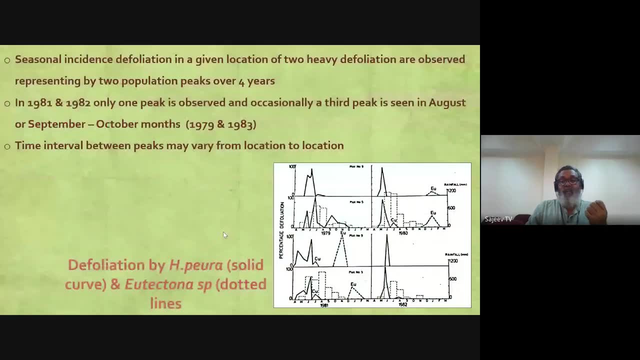 generation. There will be nearly 15 million moths per hectare to produce one generation And the seasonal incidence is depicted in the graph over here. There are cases we get a peak outbreak period And you can see over here, starting from May-June we have got small epicenter populations. And then, during the monsoon period starting from June-July, you get a big peak of outbreaks, And in some years, we get a second peak during the northeastern monsoon. Okay, Okay, I'll take a small break, one second. Hello, I'm back. sorry for that. What has actually happened is that Tea is a distance tree. During the November to December there will be absolutely no leaves on the plant, So there will be no insects found. By the pre-monsoon showers, which happens in the late February, we get the new flush. 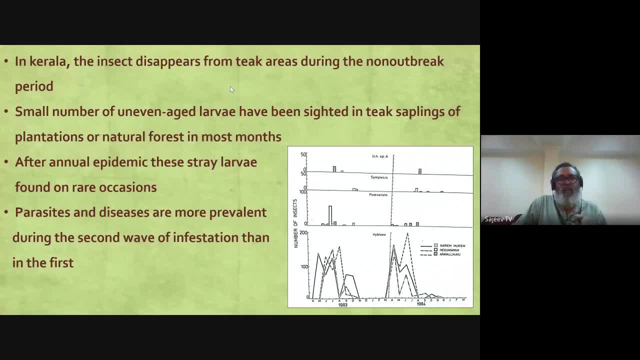 on the tea tree And by the end of February, early March, you get small outbreaks, small what we call the epicenters. It will be small in the area, Less than a hectare in the area, But there will be intense amount of. 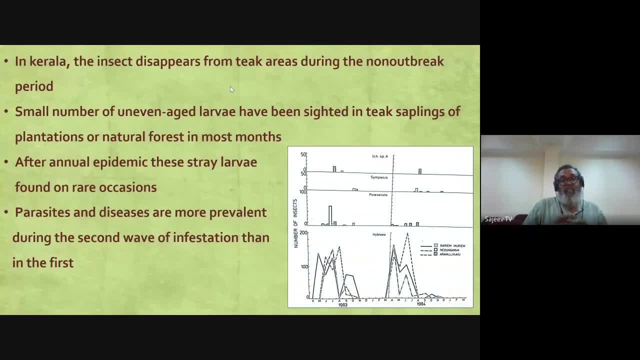 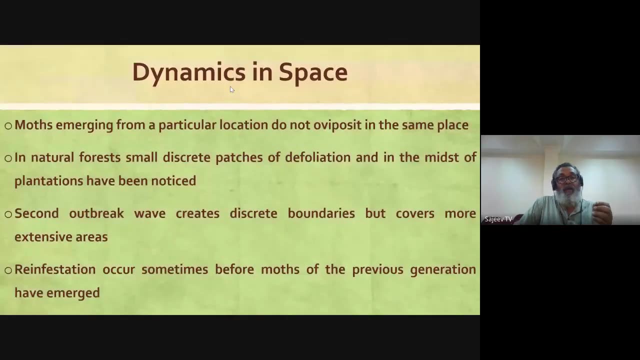 Okay, insects over there, so that's after that generation. they spread to larger areas and parasites will be very active during this particular period, but then they are not able to prevent an outbreak of the insect. and we have studied both the dynamics of the inside in both human space in time as 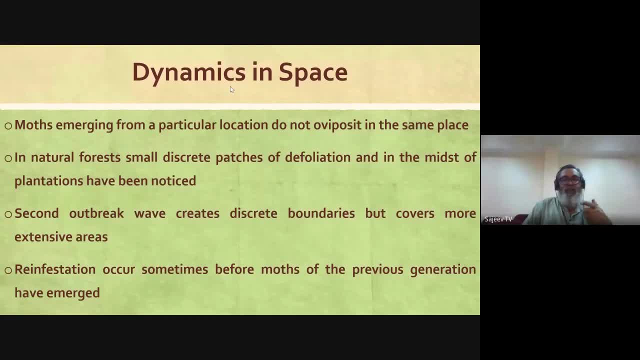 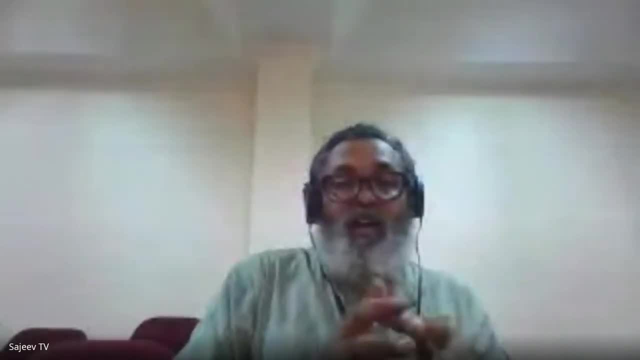 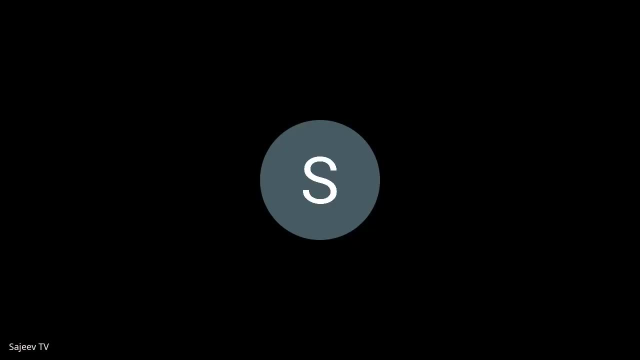 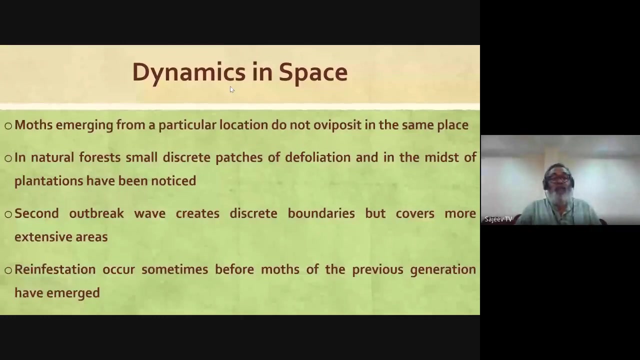 he's told earlier, i have described what happens in the temporal dimension, in space. what happens is that there'll be a small uh uh transform into uh, the uh outbreak phase, uh or the epidemic uh phase where large areas are being infested. So this is what is happening in Kerala and we have observed 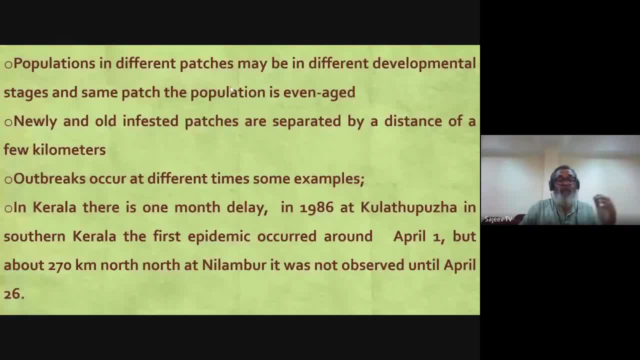 that the very first outbreaks happens in the southern part of Kerala and there is a gradual spread of the outbreaks towards north, and this follows very closely with the movement of the monsoon also. So this is about the details and this is the existing model There. 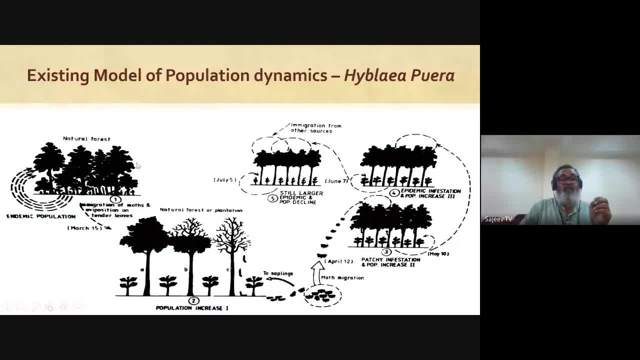 is a natural forest over here. that could be moss coming from the natural forest to start infestation in the population, and the moss which is emerging from the small natural forest or plantation can move over to the plantations and can cause patchy outbreaks. and this patchy 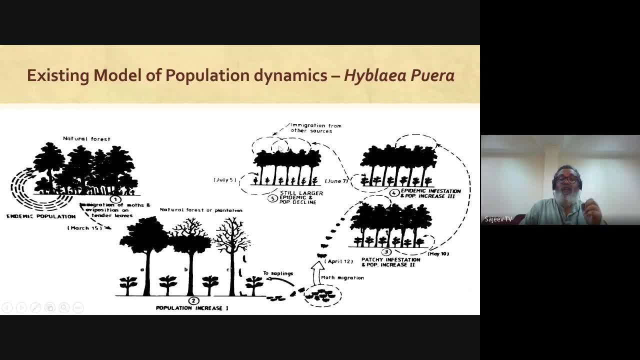 outbreaks can, in turn, lead to larger outbreaks or killing of vegetation on the tree, And our one thing which is very interesting is that whenever moss emerge from a particular site, they invariably migrate to new locations. They don't stay there, And this is one way. 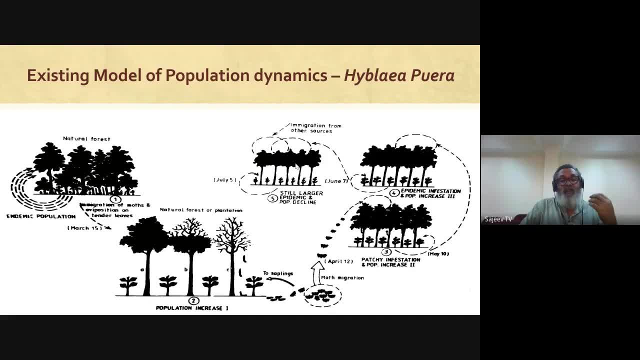 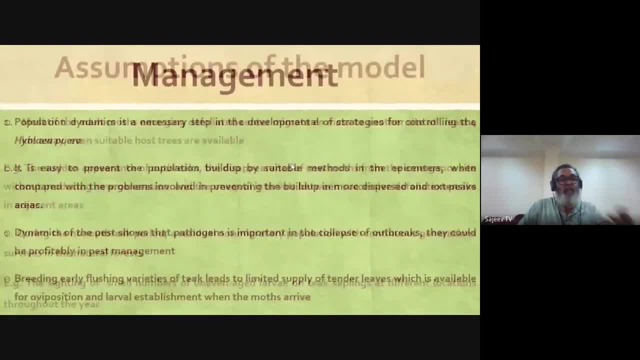 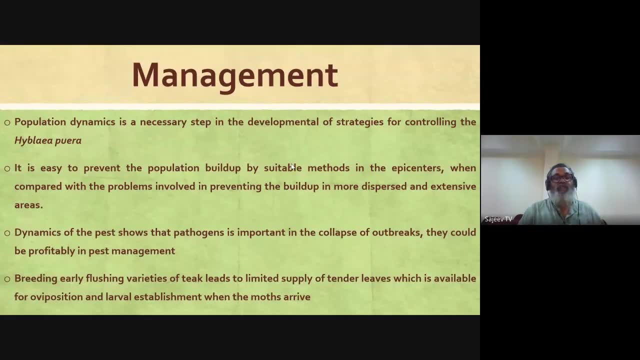 in which they have the parasite population which has been built up over the years- And I will not be going into the assumptions- And from the management point of view, looking at the population dynamics is extremely important to understand the population dynamics and how to manage the insect. For example, we have developed this particular virus which 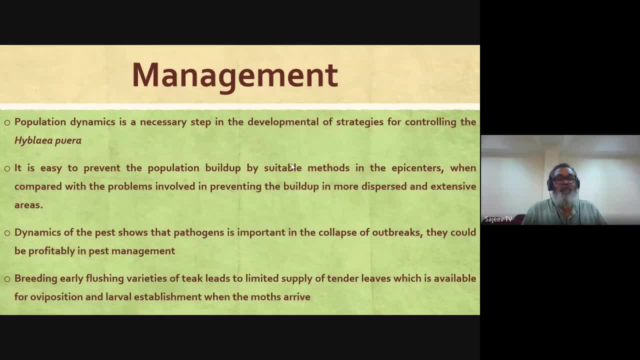 I had been explained earlier, which is a biopesticide, which is called a Hip Check. Now what we are having, a model to control the insect- is to target the epicenter population. So epicenter populations are the populations between the epidemic phase of the population, So the epicenter 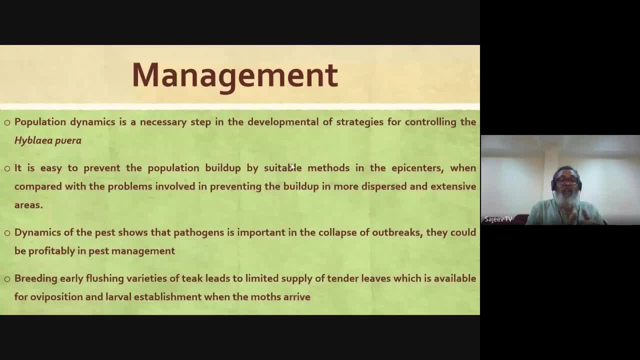 is there to deliver the virus, and the beauty of this virus is that it can. it will magnify, sprayed in the field, every insect which is imbibing, the virus or the virus multiplies within the body, and the large amount of viruses relates to the environment, so that 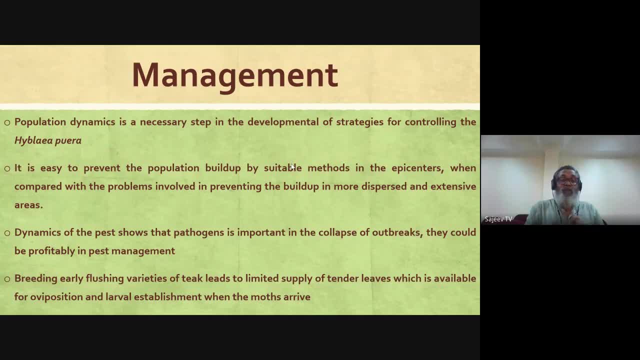 will be affecting the other insects which has been not been affected when you did the spray. so there's a horizontal transmission happening and, if ever any larvae, this doesn't get the required dosage of the virus. what happens is that it will remain and transmitted from one generation to the next generation, and so what we do is to 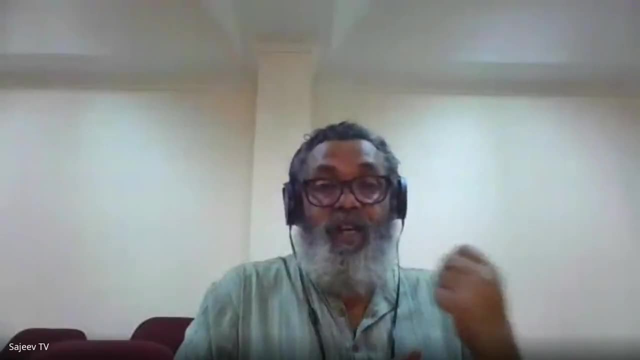 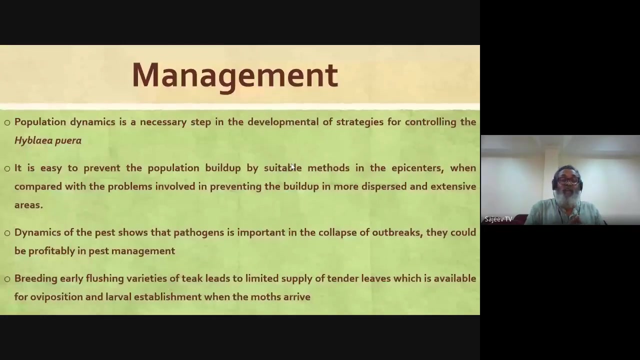 uh have a to give a uh sublethal dose of the virus uh in the epicenter population so that the moths which are emerging from that particular population becomes carriers of the virus. they will not be dead, but then there will be carriers so that whenever 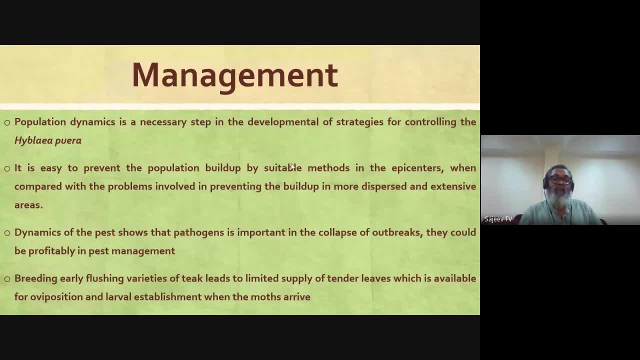 they interact with moths which are immigrating to that particular area. when they mate, the auspices will be automatically killed because of the transmission of the virus. and the vertical transmission happens in two ways. it can the virus can remain in the surface of the egg or it can be. 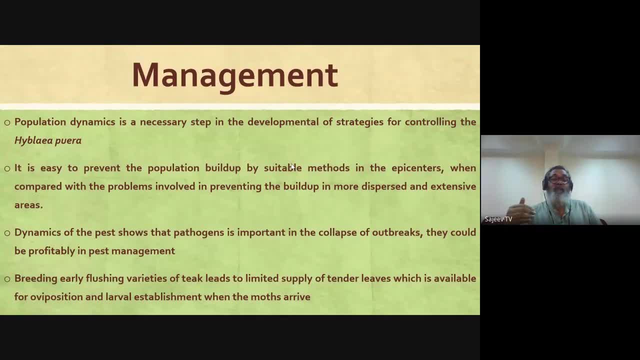 in the egg, also the transform and the transformer in modes of vertical transmission. so this is the case where the population dynamics uh helps us to uh to manage a pest to the easiest method possible, because when the big cloud place happen, it is extremely difficult to take permission because it's a large amount of area and you will have to go for the aerial mode. 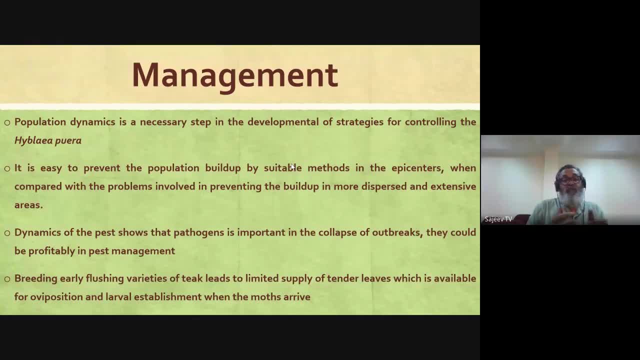 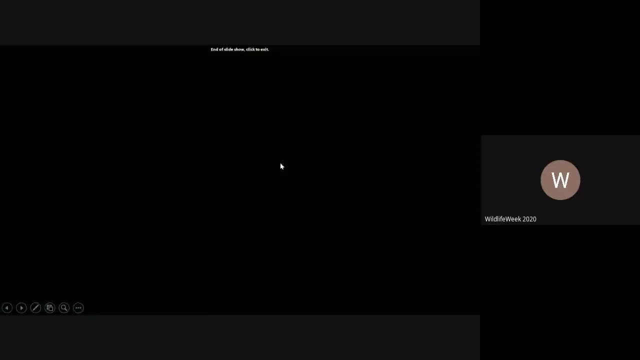 of application. but in epicenter you can do the spraying from the ground. you'll be using an absolutely safe uh target specific uh baccala virus to do the spray and you can prevent the uh inside out breaks. thank you, thank you for the patient hearing. thank you so much, sir, for sharing so much. 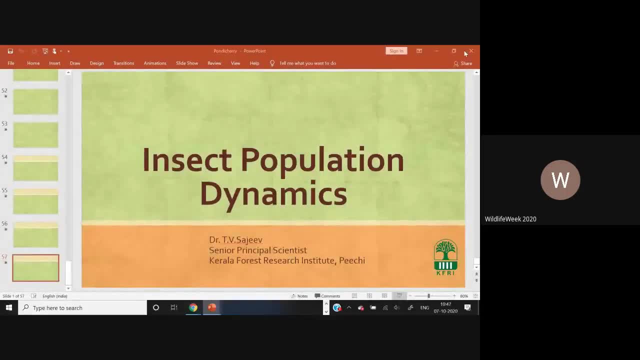 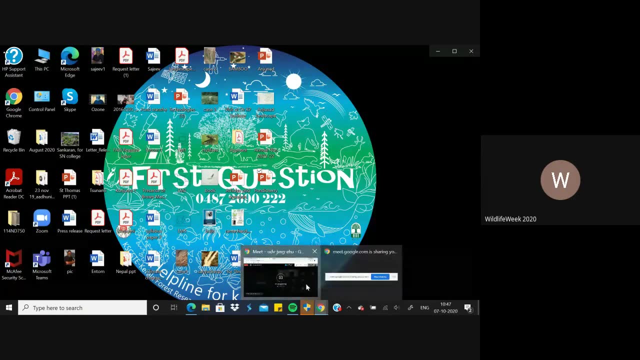 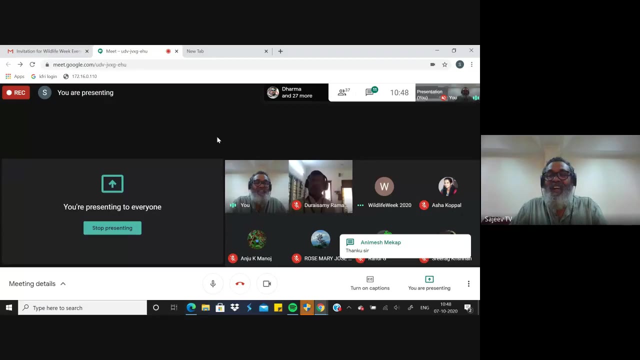 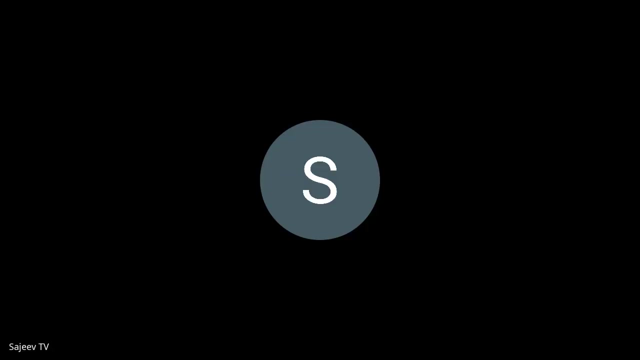 information about insect population dynamics. so there is one question in the chat box. would you like to take that question? yeah, have a look at it. what is the difference between a moth and a butterfly? oh, okay, uh, there are many very interesting uh, the agony of a butterfly. it will be straight, simple. and there's a small bulb like 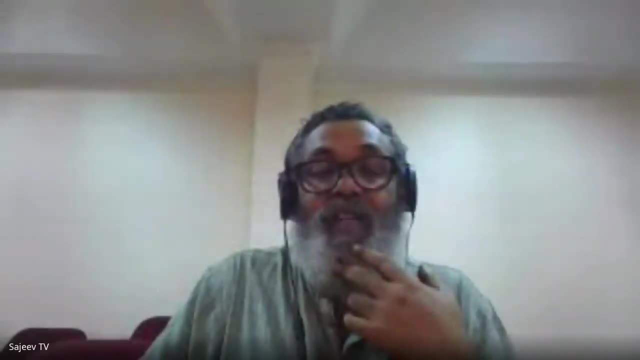 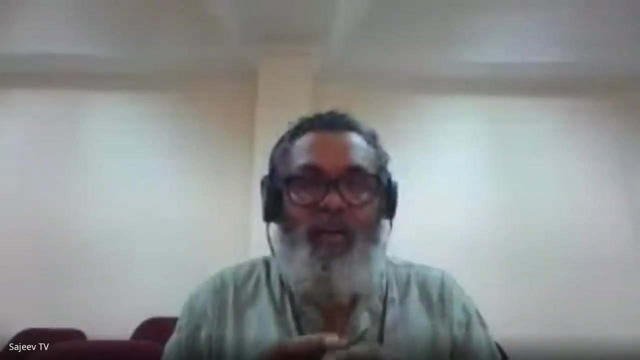 think bulge at the end of the agony. but if you look at the agony of a moth, it will be completely different. it will be just like a leaf or a or a feather. it will be branched. so the single most important criteria is to look at the antennae. There are other differences also When you see a. 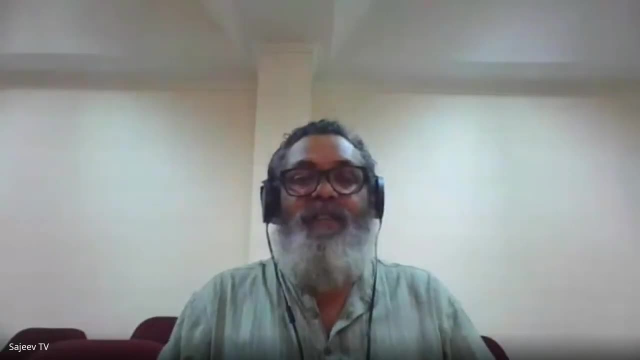 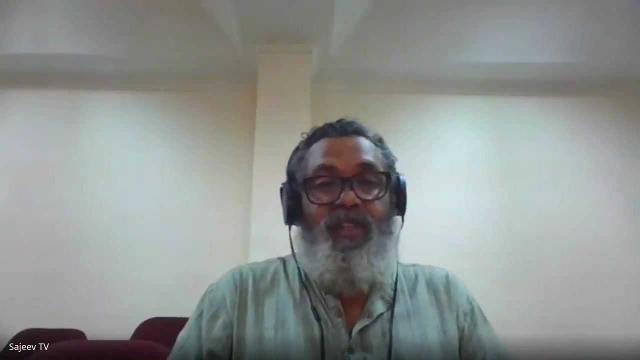 butterfly sitting on a rusting, it will have its wings spread horizontally to the ground, but when the moths are there it will be closing the wings on top of them, And moths are generally dull colored and butterflies are brightly colored And moths are quite active during the. 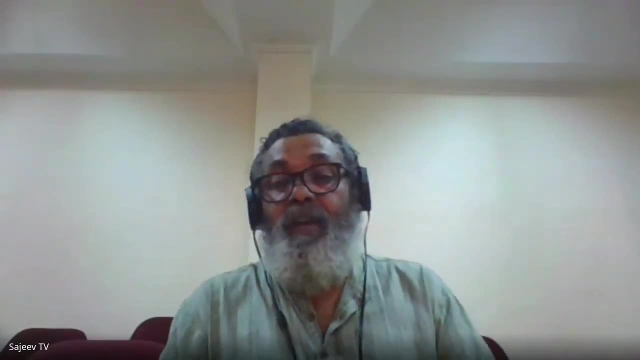 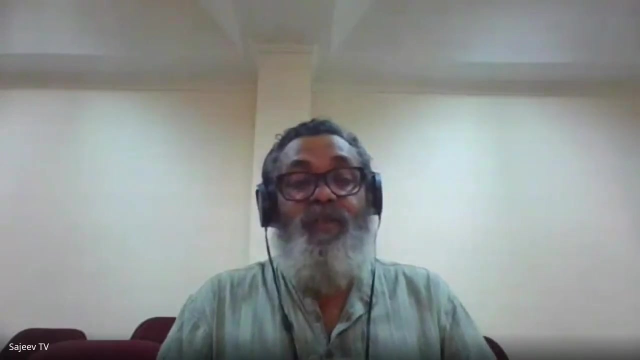 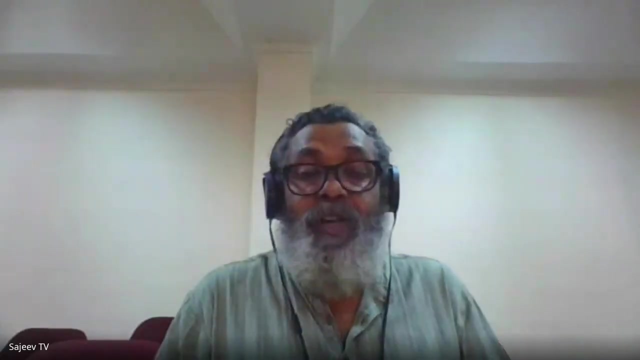 night and butterflies are active during the daytime. But then watertight compartment there are other groups of. there are some group of insects which have got the characters of the butterflies and the moths, especially the group called skippers, a group of insects which come under the group Hesperidae, So they are basically 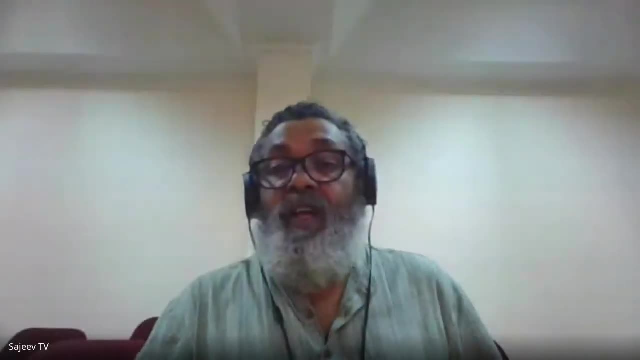 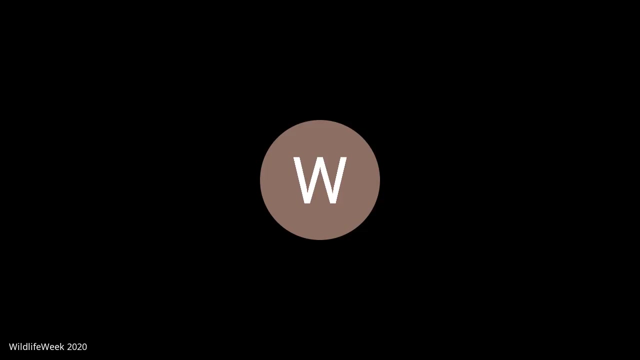 having characters of both the groups. I hope I have answered. Yes, thank you so much. So we'll not be taking any more questions because you are busy today. So thank you so much for taking out your time, taking out time from a busy schedule. So thank you so much. on behalf of the. 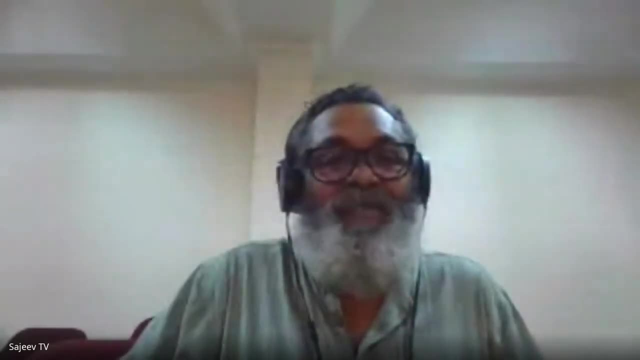 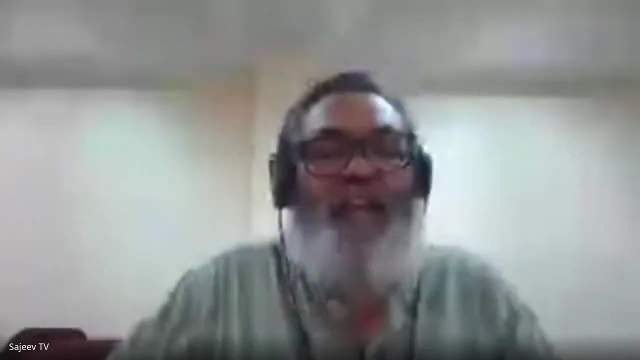 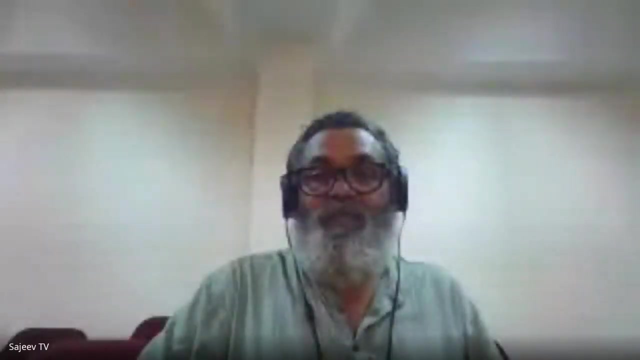 Ecology and Environment Science department. Thank you for the opportunity. Best wishes. Thank you, sir. Thank you, Thanks to all participants. If you have any questions, you can send it to us. I'll send it to Sajeev sir. He will answer. Thank you so much. 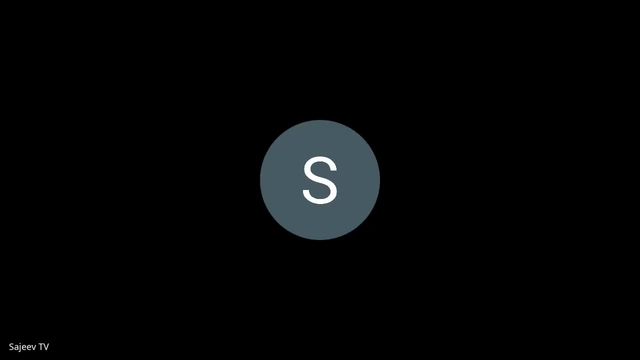 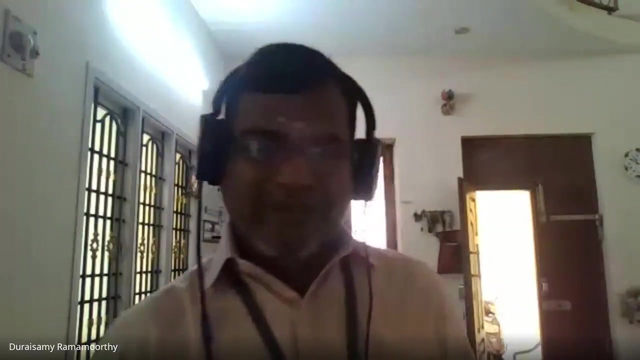 Yeah, that's good. I'm extremely constrained over time, Sorry for that. So any questions you can mail me. You can access my email ID from Abhinav. Thank you all, Good sir. Thank you, You're welcome, sir Abhinav. 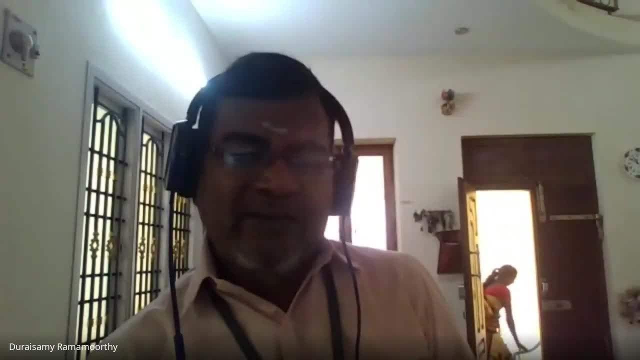 Yes, sir, Okay, I'll meet you in the afternoon, okay. Okay, sir, Thank you, Okay, Take care. Thank you, sir, All the very best. Thank you, sir. I hope you have a good day. 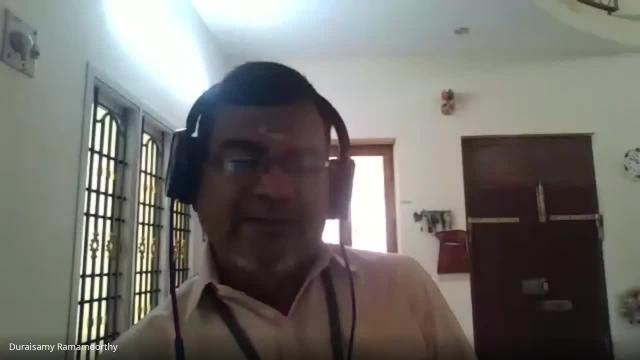 Most welcome. Most welcome. Thank you, sir. I'll drop my email again. Thank you, sir, For the certificates. Okay, See you tomorrow with another new session. Thank you, No, no, Today at 2 o'clock, no Another session. Take care, All the very best. 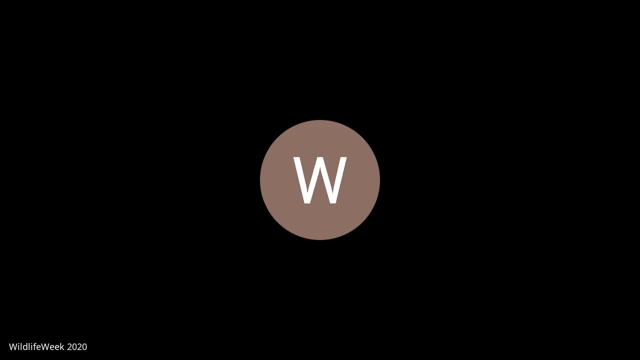 Bye, Bye, Bye, Bye, Bye, Bye.